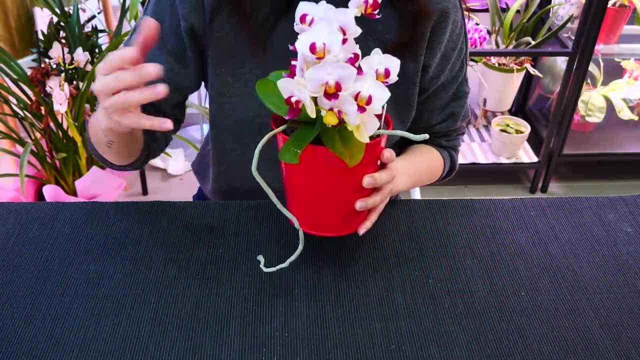 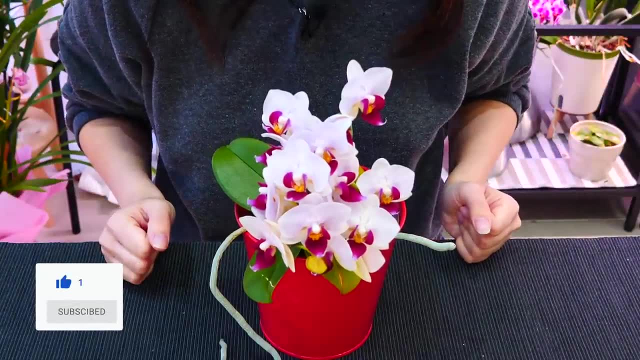 pretty good list that I hope will help most of you home growers. And before we start, don't forget to give this video a like if you end up enjoying it. It really helps it out, And why not subscribe? I post multiple times a week, Right, let's start The first orchid, which I consider to be the 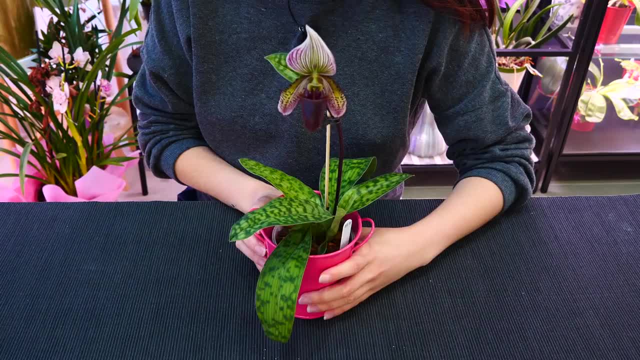 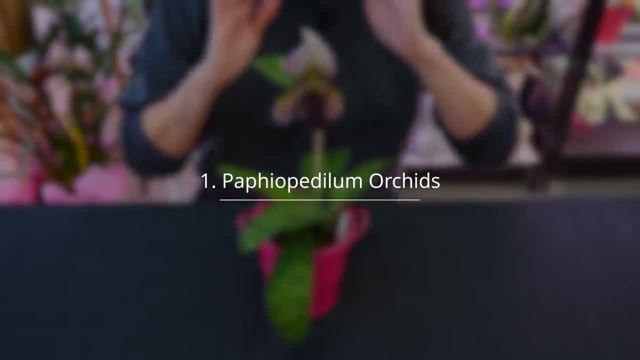 easiest to keep in a home. it's not the Phalaenopsis. It is, though, ta-da, the slipper orchid, not any slipper. the Paphiopedilum Fragment piniums, different type of orchid, which I will not address today because I really don't. 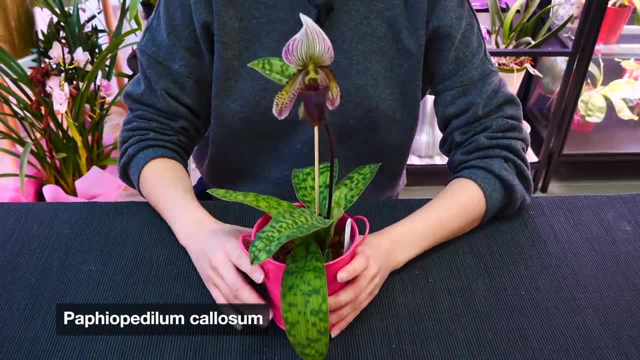 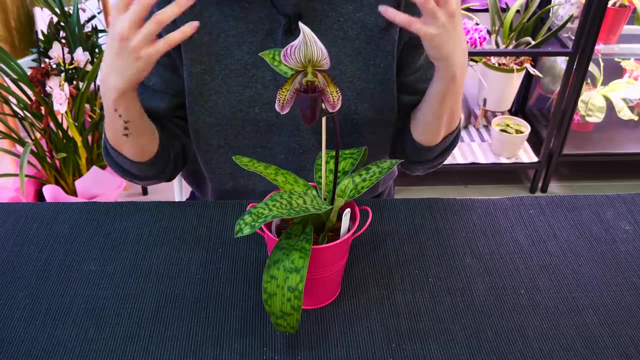 have good luck with them, But Paphiopedilums, in my opinion, are the most hassle-free orchid for home growers. Some might disagree, Some might say no Phalaenopsis is, But I have some reasons to. 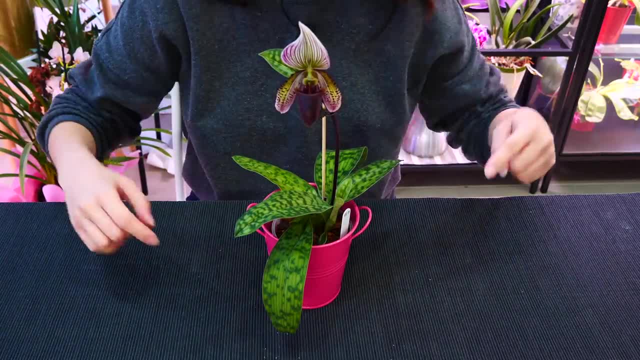 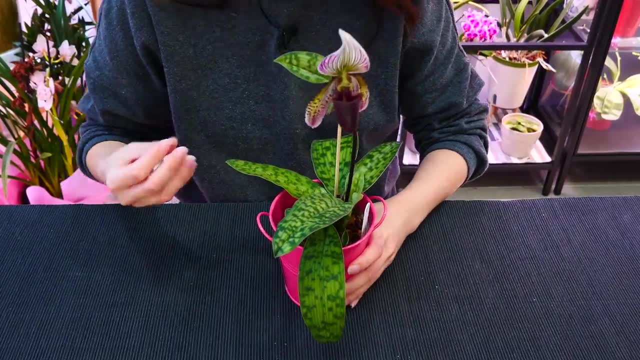 believe that again, generally speaking, these guys will not give you as many headaches. The first concept to grasp whenever we're growing most other orchids which are epiphytic is the fact that they are epiphytic. They will not behave like other houseplants. 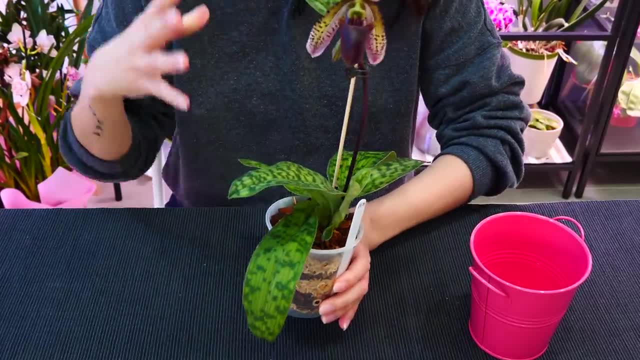 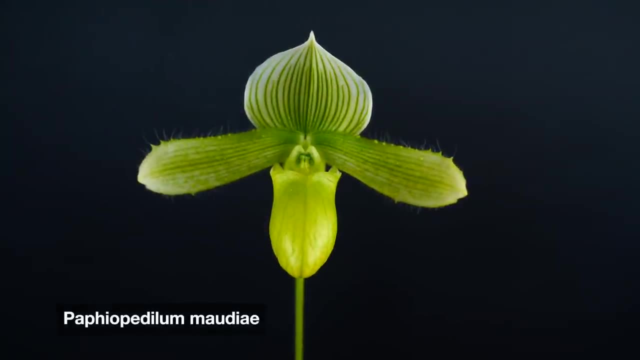 The Paphiopedilum is terrestrial so it will actually be a little bit more similar to the other houseplants we might already grow. I would say it is the in-between nice transitional plant, because this guy doesn't really like to dry out, So it is much more forgiving to more frequent 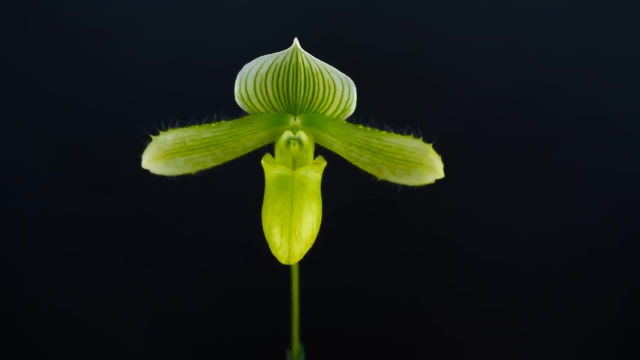 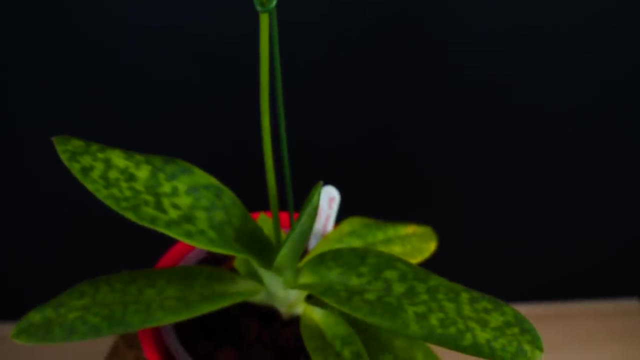 watering to, let's say, more of a denser substrate. This is not the type of orchid to put out aerial roots, And most of the times you won't even find it for purchase in transparent pots. So, first off, I really don't think it's as intimidating. 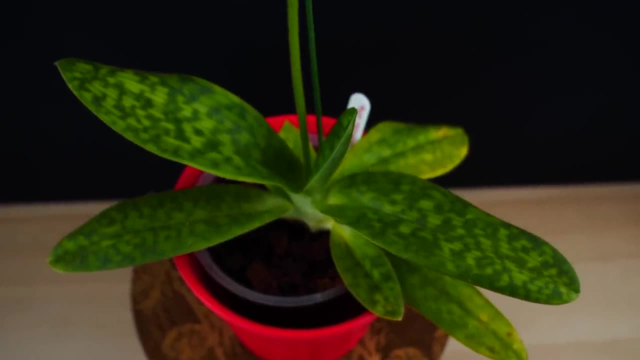 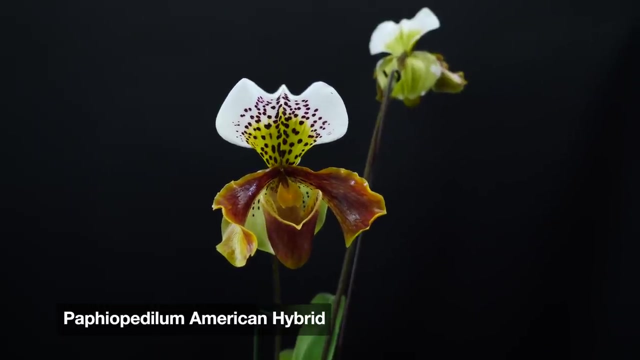 As your first Phalaenopsis might be, with all the transparent pots and roots everywhere. Second, when it comes to care requirements, it doesn't really ask for much. It doesn't even ask for bright light. Temperature-wise, it is comfortable in a wide range of temperatures. 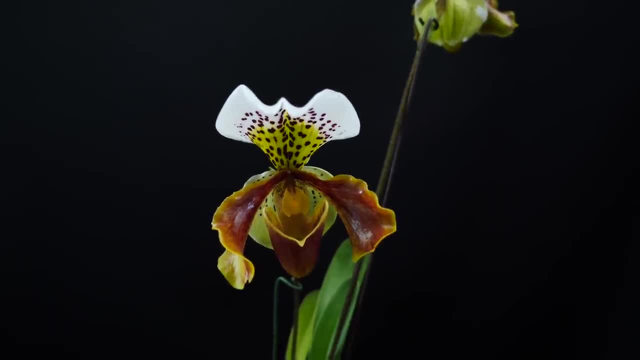 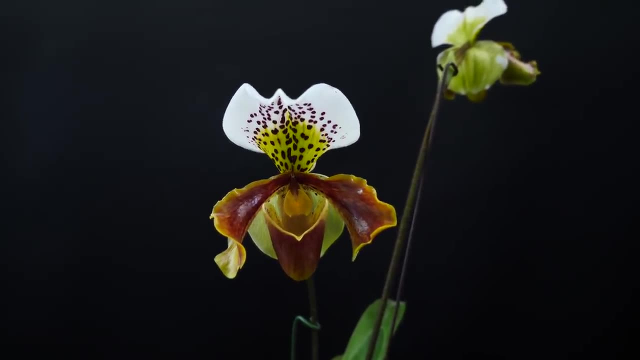 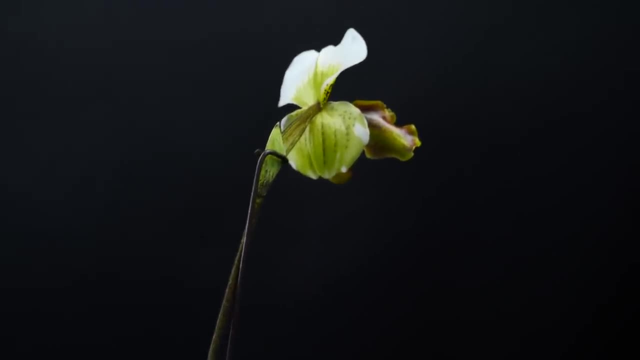 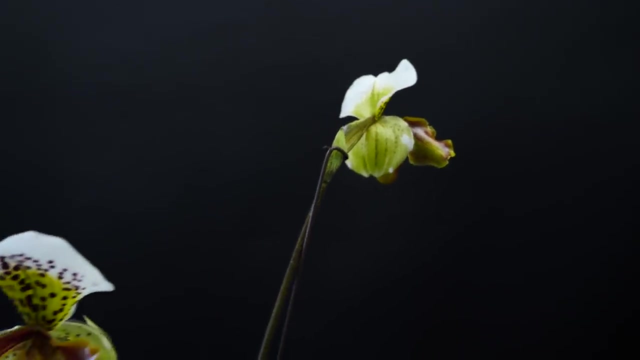 I think it's a good idea to give it a try. I think it's a good idea to give it a try So it might actually bounce back with a new growth Bonus. it looks so, so pretty. Yes, it's not going to be in bloom for as long as a Phalaenopsis not going to have all that beautiful. 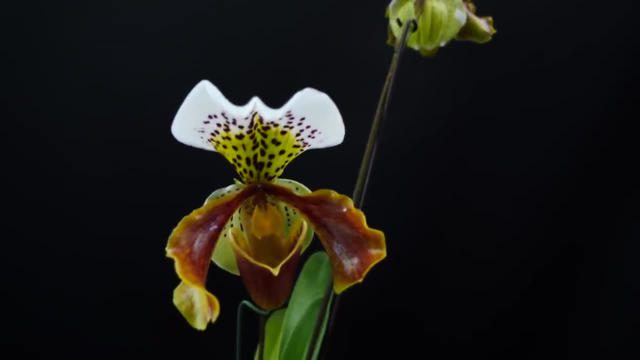 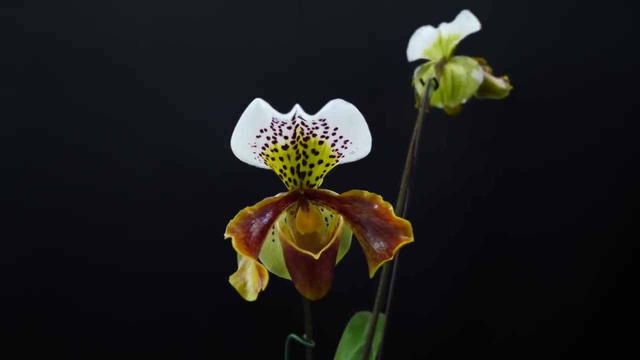 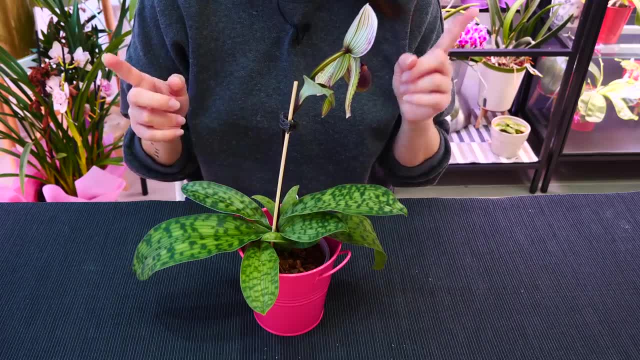 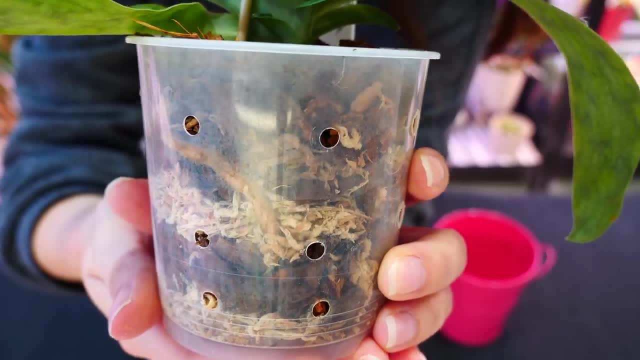 office lighting situations, not to mention. they are quite resilient. Yes, they don't really like to dry out, but I don't know, if you noticed, mine is very dry. I'm late with watering day. It has been a busy week. Do you see him wilting? No. Do you see the flower fading? No. So yeah, he doesn't. 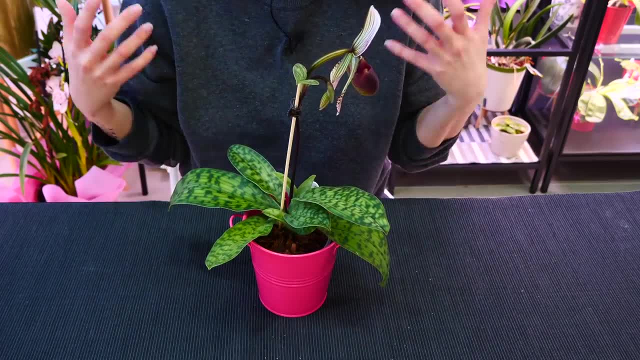 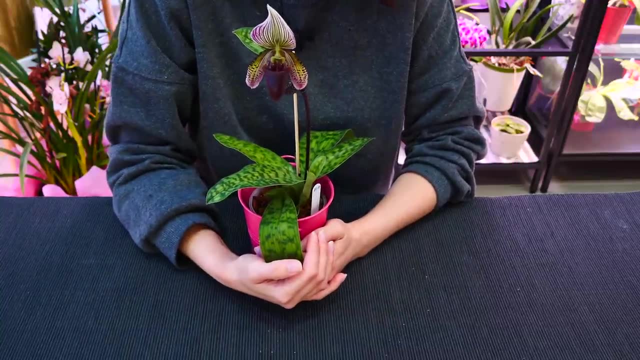 like drought much. but if you just have a busy day, if you postpone watering a day or two, he's just not going to mind it. He's going to completely understand you And for that reason I really love slippers. I really do. I find them easier than Phalaenopsis Orchid number two, the Phalaenopsis. 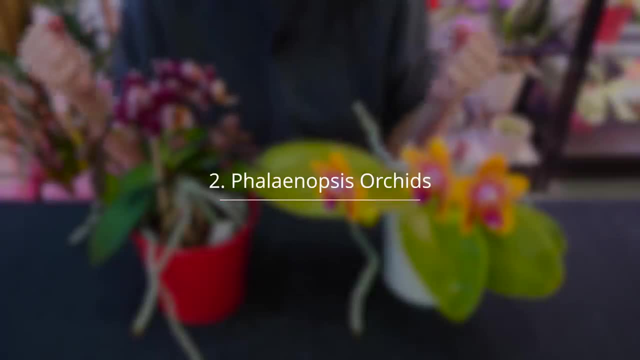 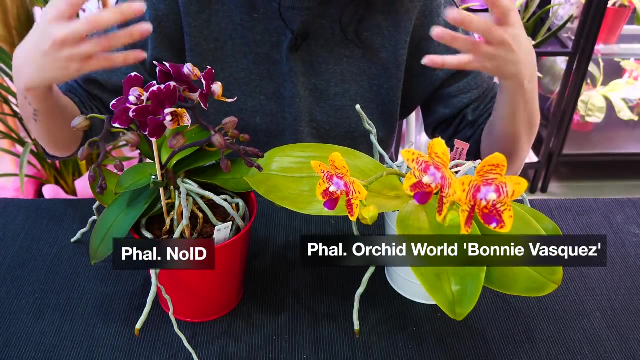 Even though, yes, it has its soft spots and sensitivities. but you know what, Throughout the years, anywhere that I lived, I have been more consistent with Phalaenopsis success than any other thing, And you might already know, Phalaenopsis are the most popular orchids. 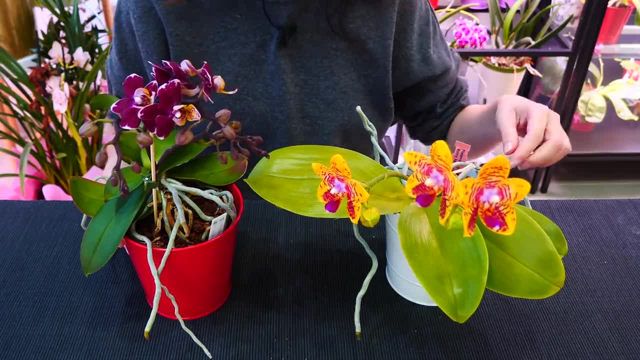 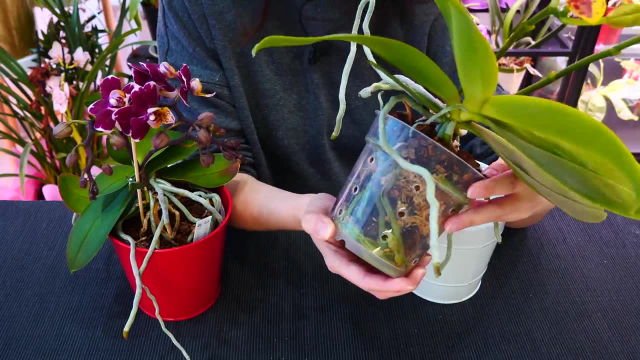 and that's for a reason. Now, Phalaenopsis are epiphytic orchids, So the thing you need to get used to the most is the fact that they don't like to have roots that suffocate. They need a different type of potting mix, maybe a different type of pot, a transparent pot. They will teach. 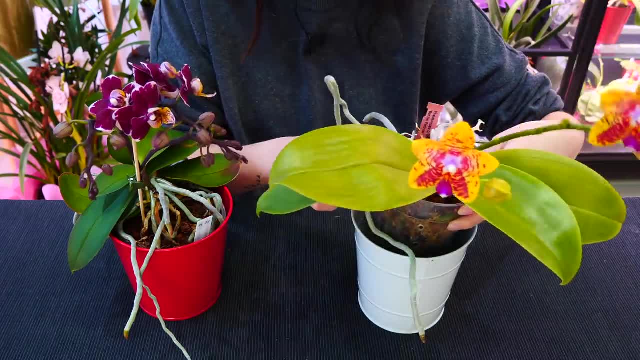 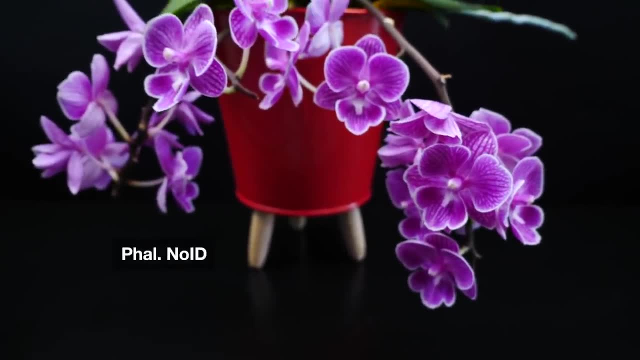 you patience, because in order to rebloom them, you need to be patient. You need to grow them vegetatively. You might do a few mistakes along the way, like rotting the roots, rotting the crown or the stem. Yeah, there are all of those things happening, But with other orchids I feel like 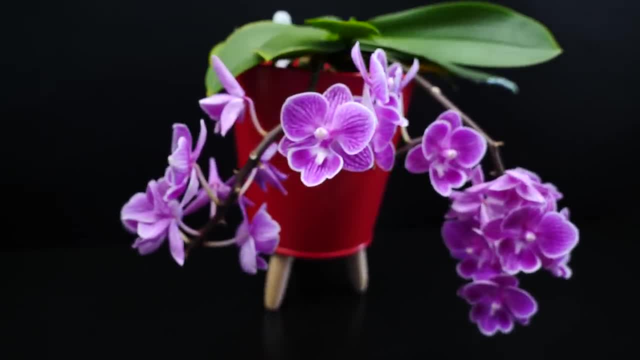 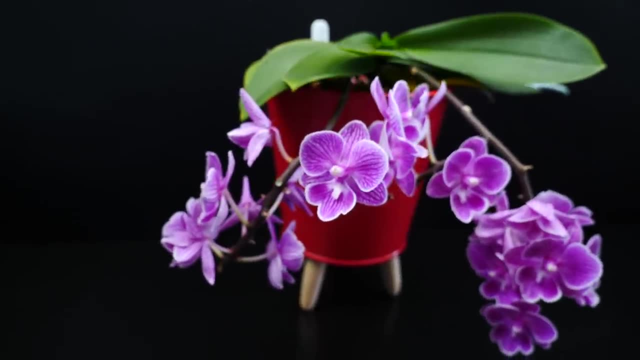 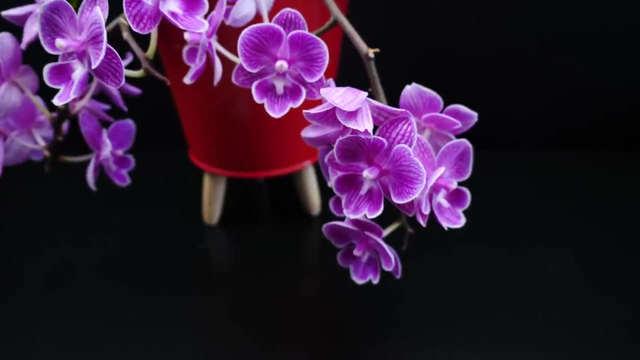 there are worse things that can happen easier for home growers, And again, in most countries they are very affordable as well. But what I believe is one of the major drawbacks of these orchids is that they have a little bit of a trick when it comes. 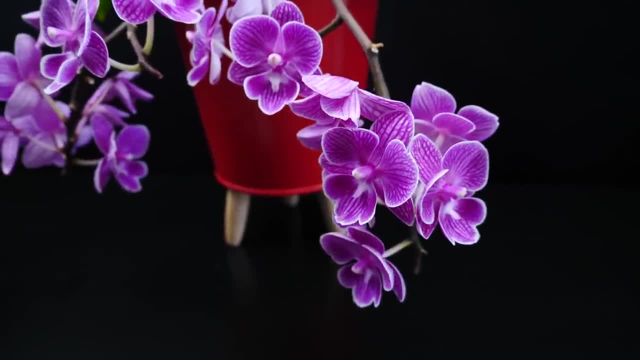 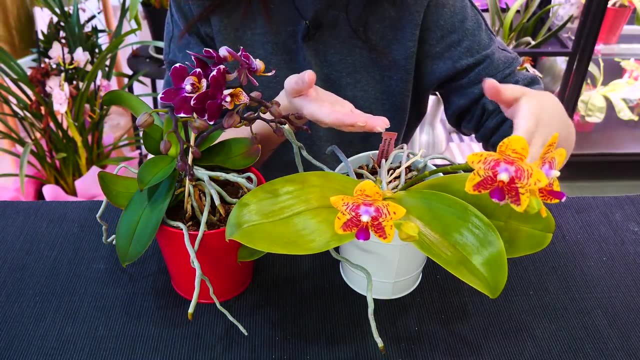 to reblooming. So, especially for those of you who live in very warm climates and have some issues reblooming Phalaenopsis, I do have the beautiful Polykylus type Phalaenopsis or hybrid, which is much, much easier to rebloom. To better explain this, I have a video that I filmed. 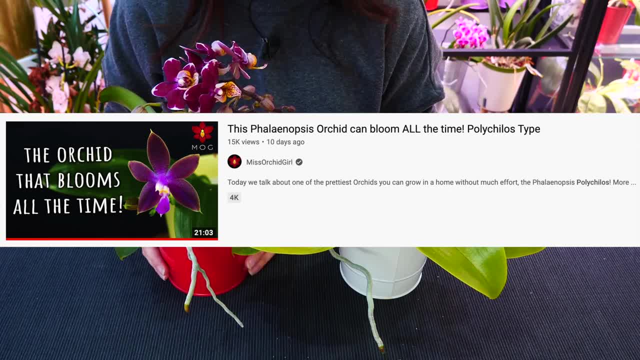 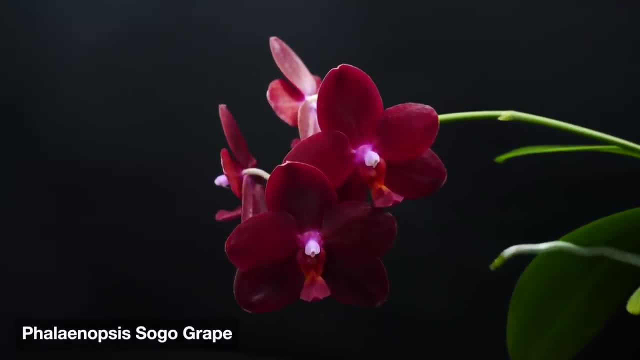 which you can check out in the description below, But online, I do believe, there is a Phalaenopsis for everyone. Now, if you did not have success with Phalaenopsis, there is something in your care, or maybe environment, that messes stuff up for you because, really, Phals are really. 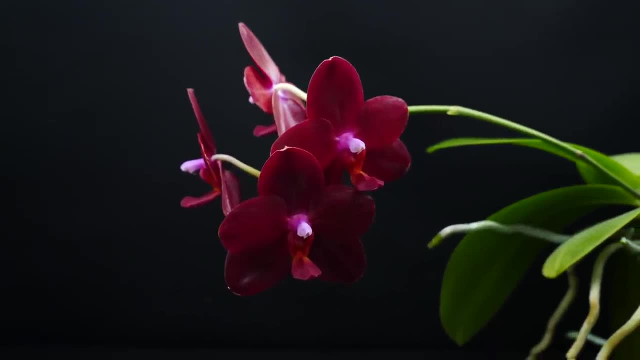 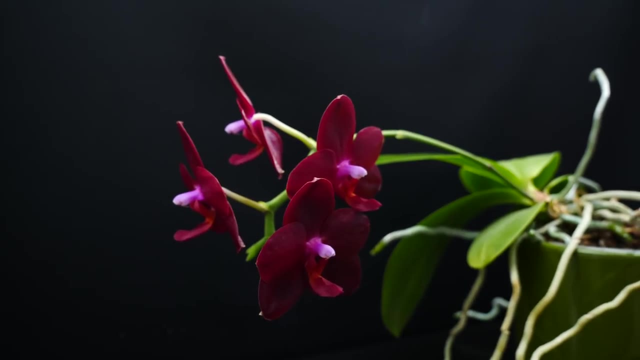 really forgiving. So try to figure out what messes up your plans, because I'm sure if you eliminate it you're not going to have issues with Phalaenopsis. And even though historically I wasn't really a big fan of Phalaenopsis, I will tell you I love 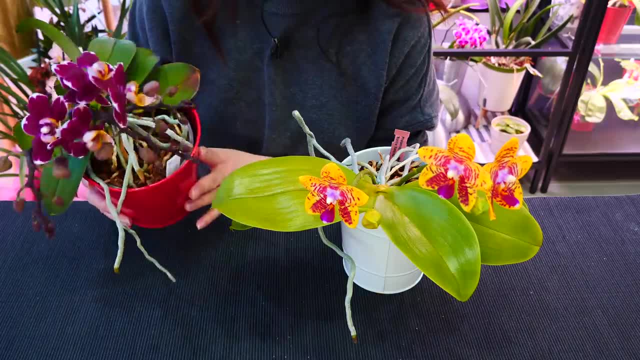 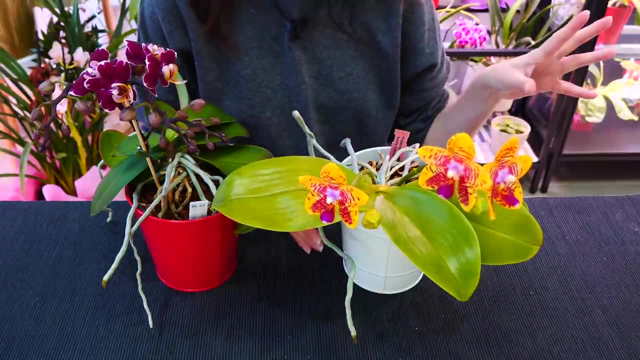 nature, Phalaenopsis, because they don't take up space and they give me the same beautiful flowers, just on a tinier version. And I also adore the Polykylus types, the Polykylus hybrids, novelty hybrids, all of those things, This thing right here, I adore it And it doesn't give me. 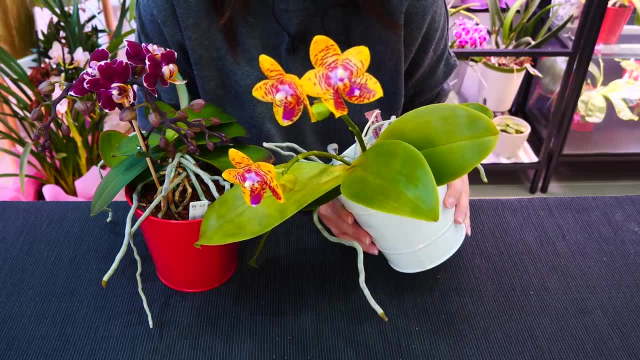 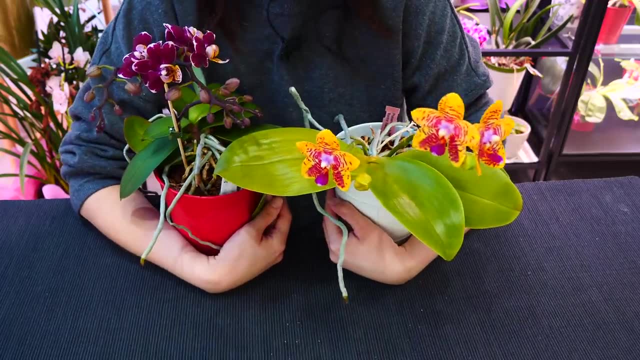 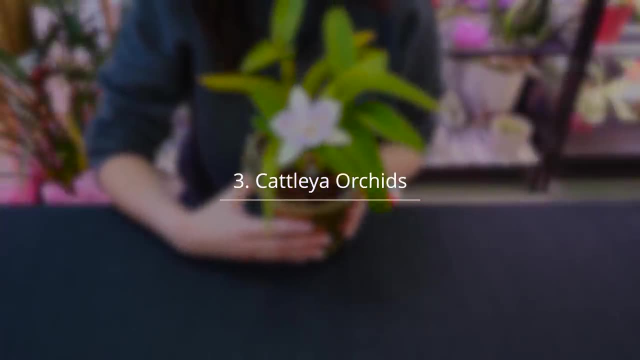 headaches quite at all. So, honestly, I'd rather focus on something like this than trying out Meltoniopsis again and failing again, you know. So these guys are my babies and I would recommend them to anybody. Orchid number three: Catlea orchids- some of my favorites. These orchids have regained some of 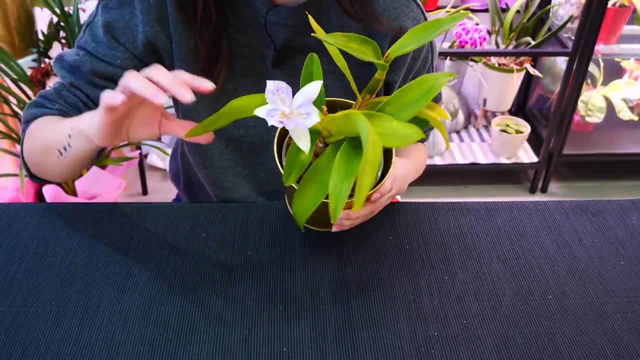 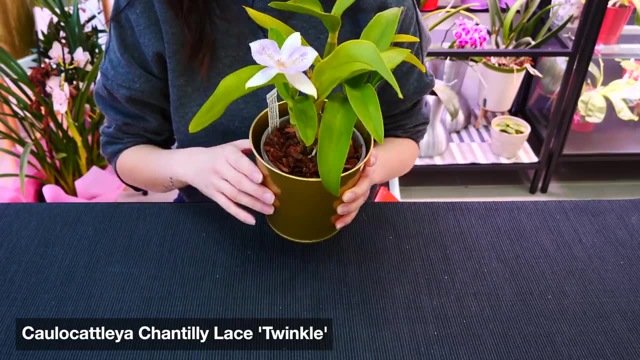 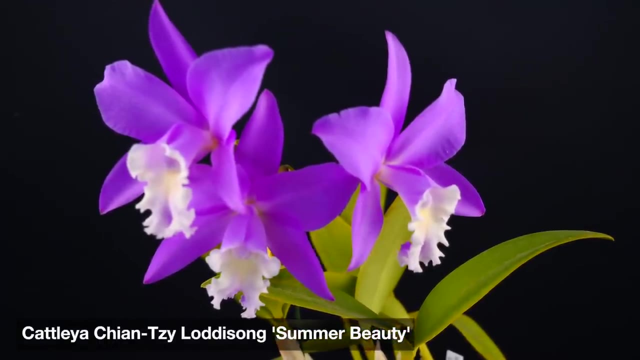 their lost popularity, I feel like in the past few years. Did you know? these guys were super popular maybe in the 40s, When the flowers were used as corsages. they were the Phalaenopsis of their time really. And well, with the availability and diversity of Phalaenopsis they kind of lost. 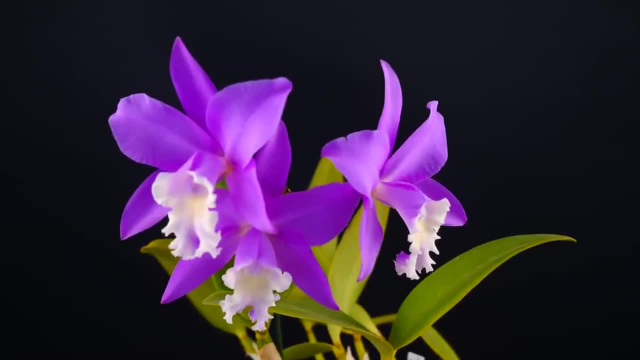 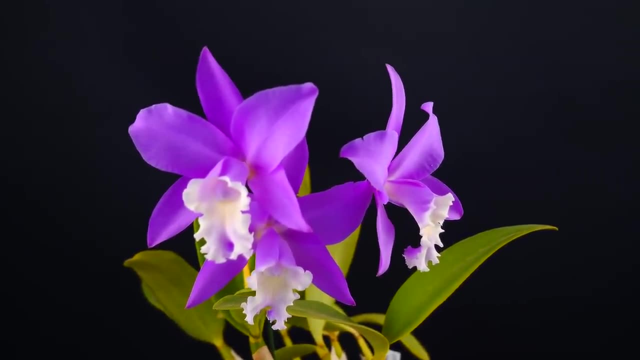 some of that popularity, but it's back. Catleas are absolutely fantastic. There are so many different types of Catleas and hybrids on the market nowadays that you can find something to suit you. If you want fragrant, you're going to. 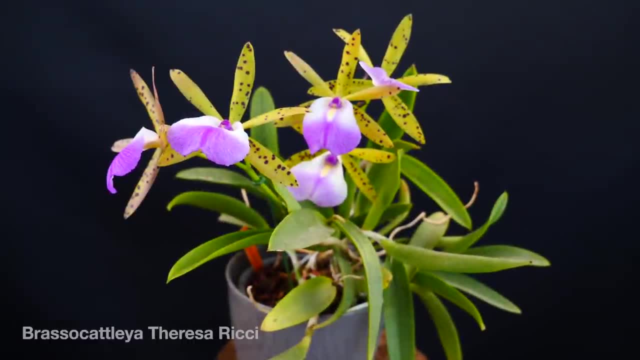 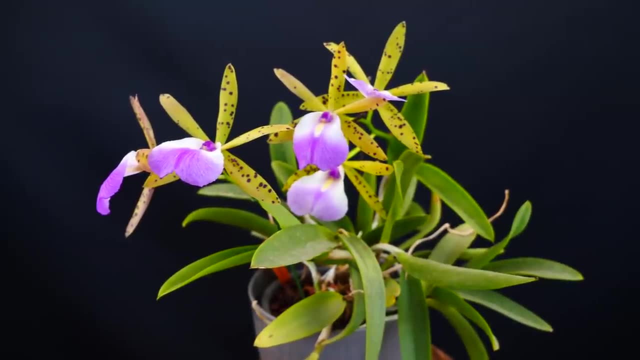 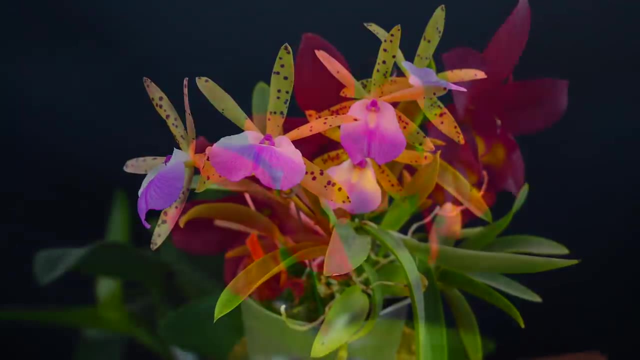 find fragrant. If you want non-fragrant, obviously you're going to find non-fragrant hybrids. Whatever color you can think of, mine is maybe black. you can find a Catlea with that color. I would love a black Catlea. Bonus: they are sympodial orchids. They are not prone to crown rot or stem rot. They 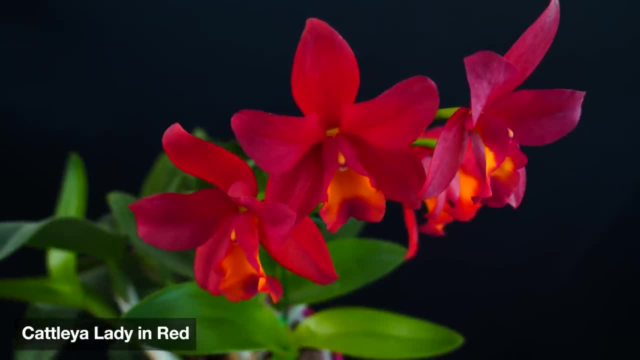 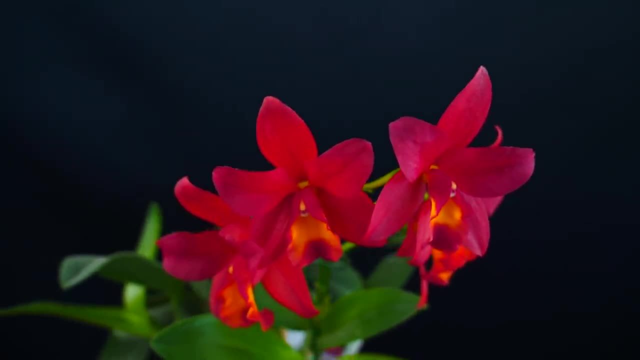 have other soft spots. They are not prone to crown rot or stem rot. They are not prone to crown rot, But certainly I do believe it's easier to rebounce a Catlea which has a rhizome rather than a monopodial. The downside of these guys is that there are so many different varieties that you 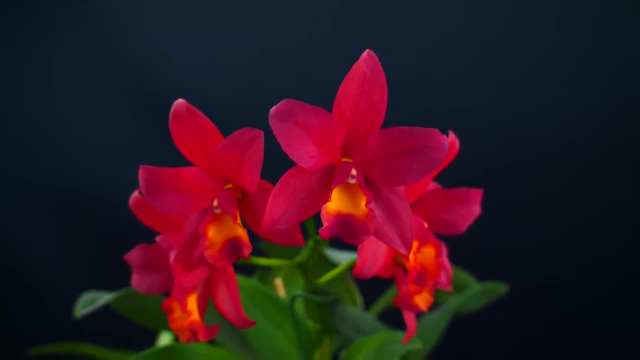 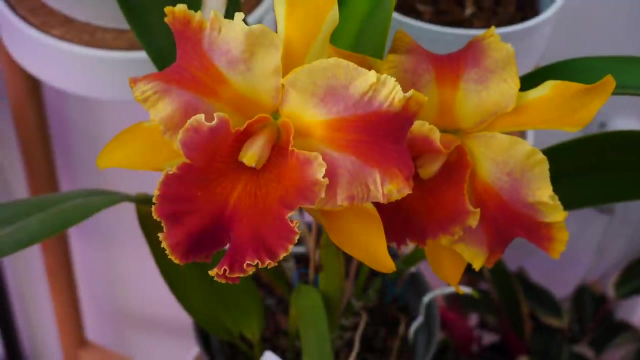 don't know what you're going to get. pretty much The hybrids are more likely to bloom more for you and grow faster, but there are some species which have terribly slow growth, species which you kind of need to time or repot of because of their very strict pattern of growth. If the Catlea skips. 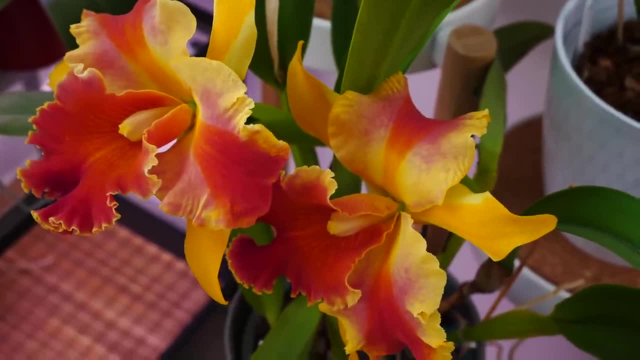 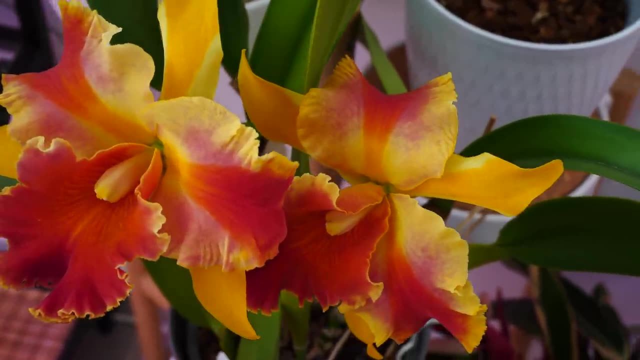 blooming this year, then it's goodbye until next year. You know there's no other possibility of it blooming this year. It can be a little frustrating with the species and maybe simple hybrids. They're also more drought tolerant. These guys are very, very suited for very hot climates. 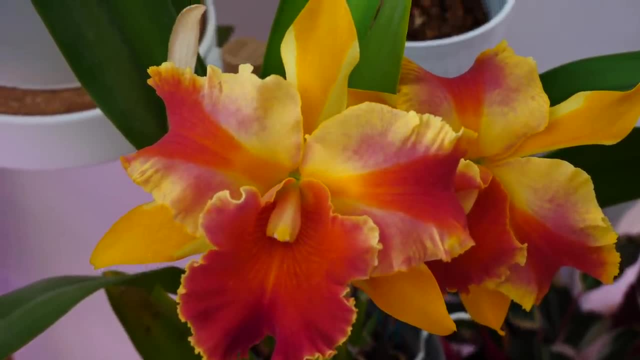 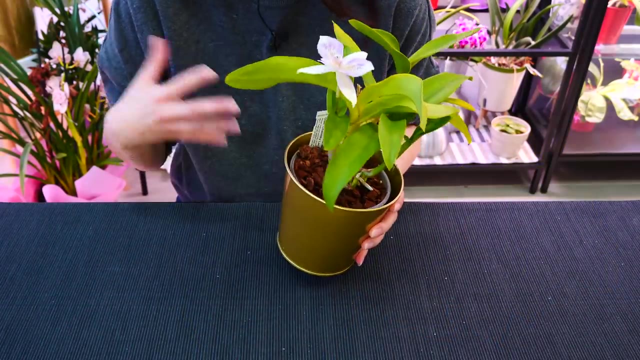 As long as you have bright light, whether artificial or natural, you should be good with these guys And really honestly, I don't think there is an orchid that can compete with the fragrance of Catleas generally, Not even Phalaenopsis, and I love. 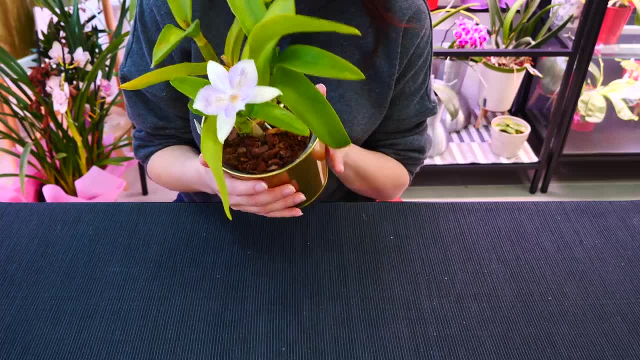 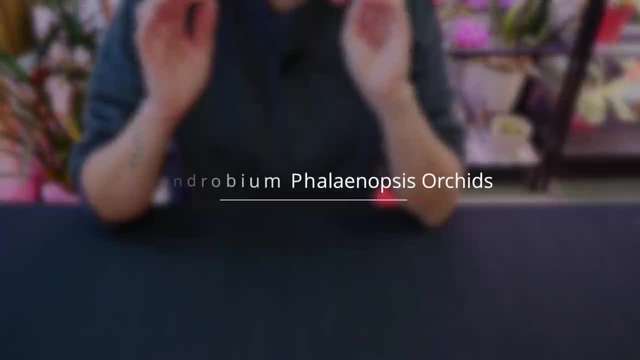 my Bellina. No, this is beautiful, I love my Chantilly, So the Catlea is third on my list. No surprise there, Fourth orchid, and I'm pretty sure I'm going to stop counting at this point. I don't have it here, but I would put the Dendrobium Phalaenopsis type orchid And this: 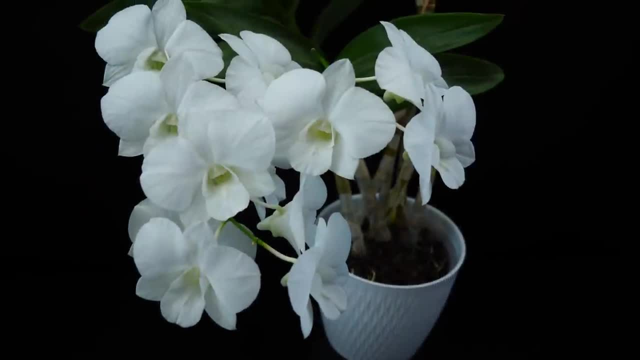 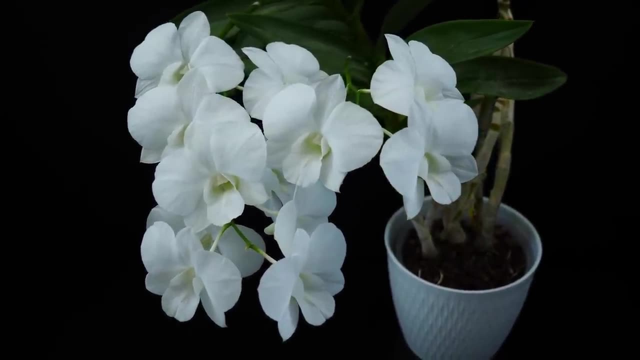 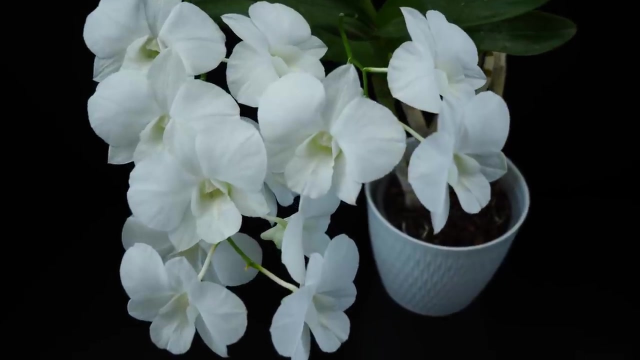 is because to me it is another version of a Catlea that looks a little different And obviously it's a completely different genus. but I feel like the care for Catleas is identical to the care of Dendrobium Phalaenopsis types, And in some parts of the world they are so, so incredibly. 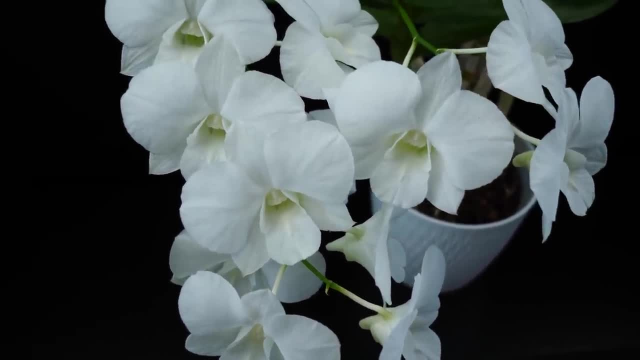 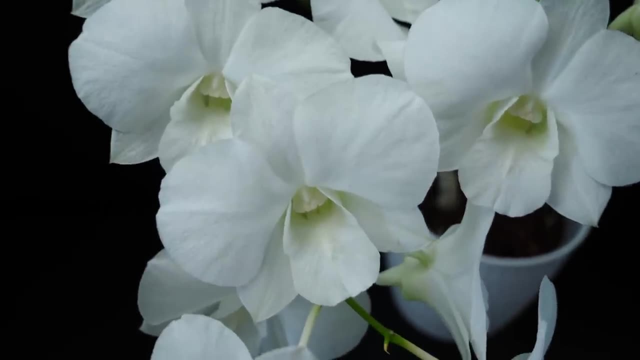 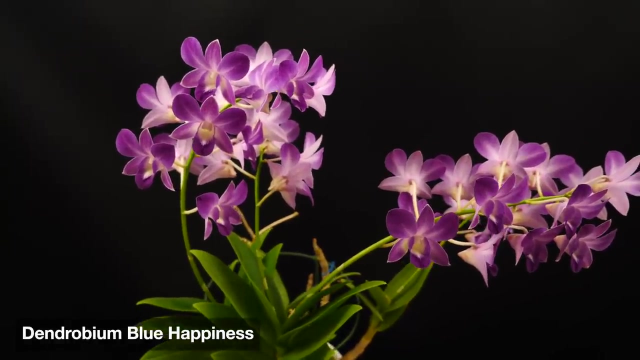 popular, especially in Asia and maybe in Central America. Am I wrong? Let me know. I feel like those climates are very, very suited for these orchids. They are hot growers, They like a lot of light. They are very drought tolerant. I don't know which is more tolerant: the Dendrobium. 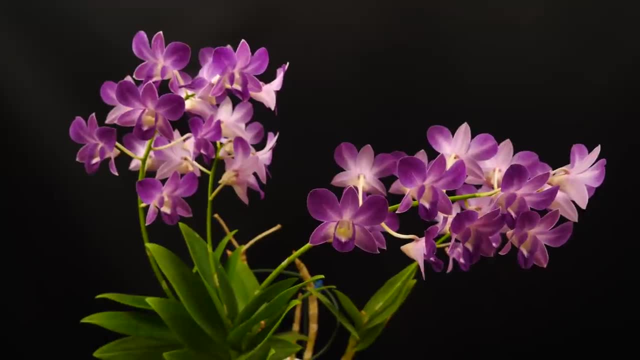 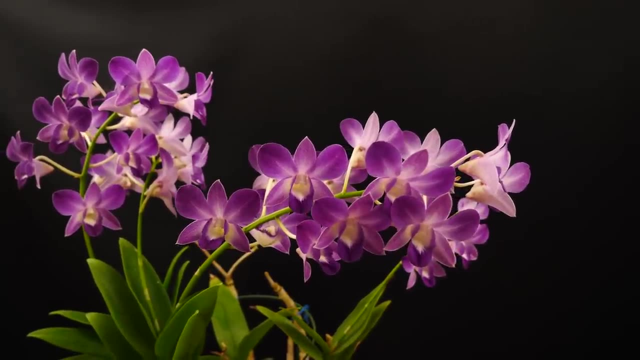 Phalaenopsis or the Catlea, but I can assure you that Dendrophils don't necessarily have a lot of need to be repotted at a certain time of the year. I rarely ever lost a Dendrobium Phalaenopsis, So 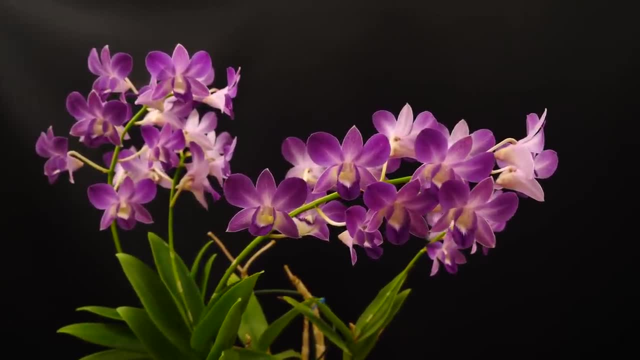 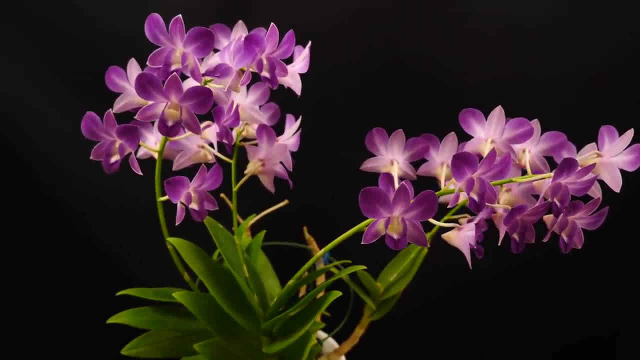 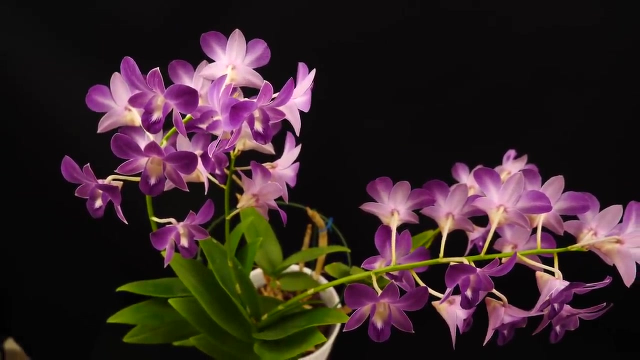 I was tempted to put them above Catleas on the list, but I won't, simply because there isn't as much variety as the Catleas. With the Catleas you can find tiny little specimens for smaller homes, smaller shelves, smaller offices. With Dendrobium Phalaenopsis types, typically you go big. 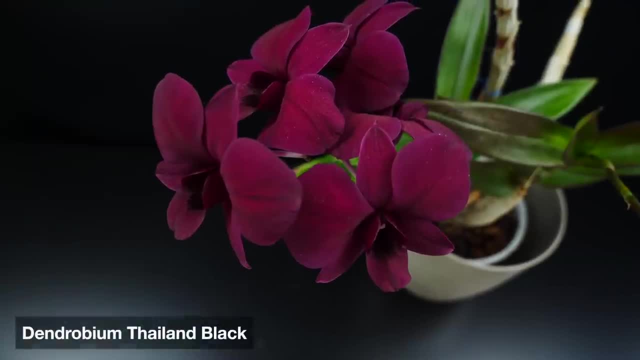 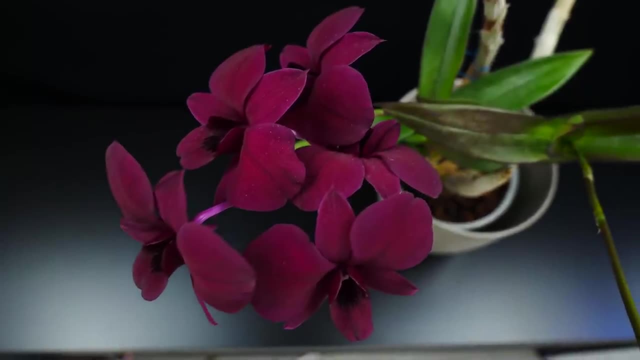 you go tall. There are very few which are actually tiny, and certainly they're not as tiny as tiny Catleas. So I find generally Catleas a bit more versatile when it comes to maintenance, But other than that, I find Dendrobium Phalaenopsis just as easy and just as much of a joy to grow. 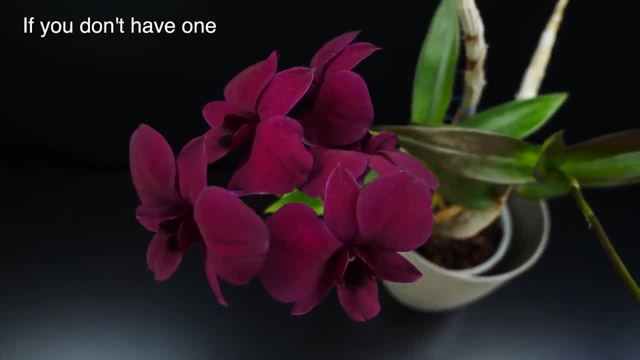 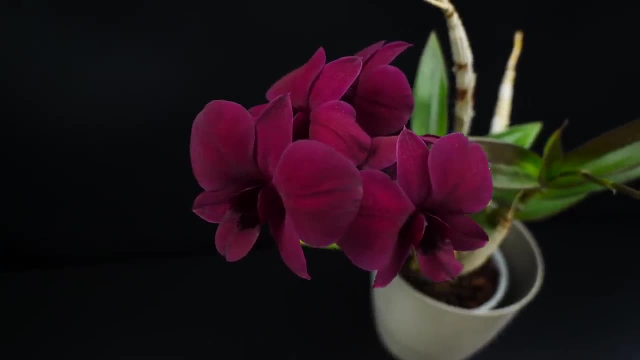 them. You might have some issues with blooming them if you don't have a lot of light, but the story is the same with Catleas as well. Anyway, to me, they're pretty much on the same level. One of them, though, is much more diverse than the other, So that's why I put Catleas in front of Dendrophils. 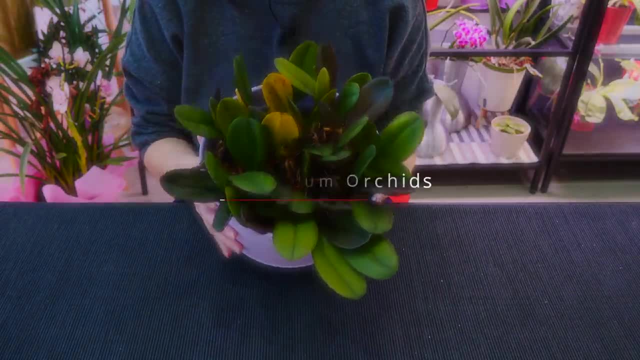 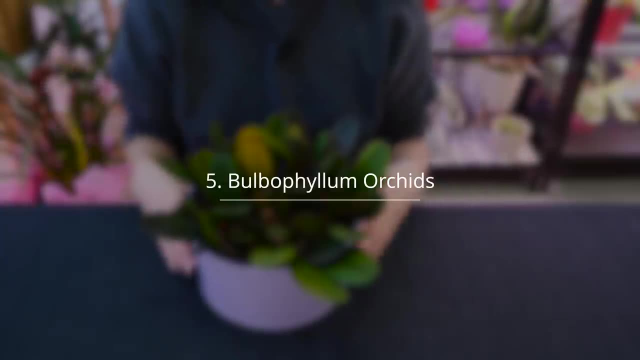 Next up more into the territory of nursery orchids, the Bulbophyllums. I love Bulbophyllums. I will get more, but the fact that they're not available at the flower shop obviously means I'm not gonna. 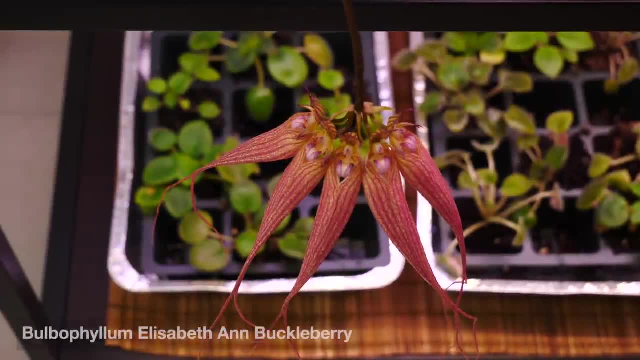 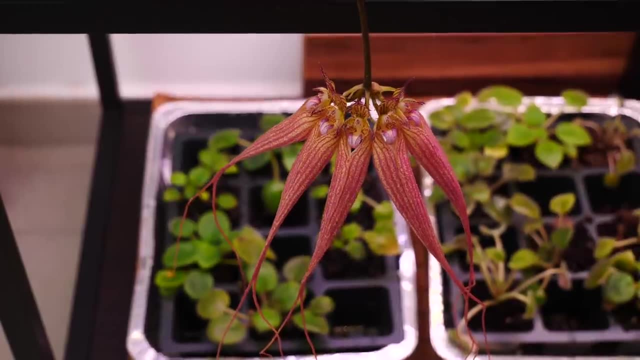 acquire them as fast. But Bulbophyllums, in my eyes, are just as easy to grow as Phalaenopsis. They don't require a lot of light, They don't require special conditions. You can grow them out of a greenhouse, just like all of these orchids. I mainly specialize in home approved orchids, So things that 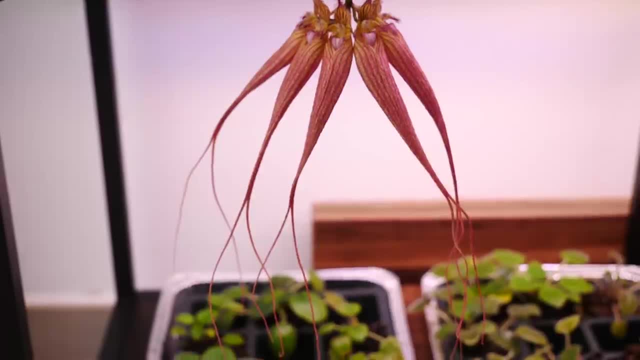 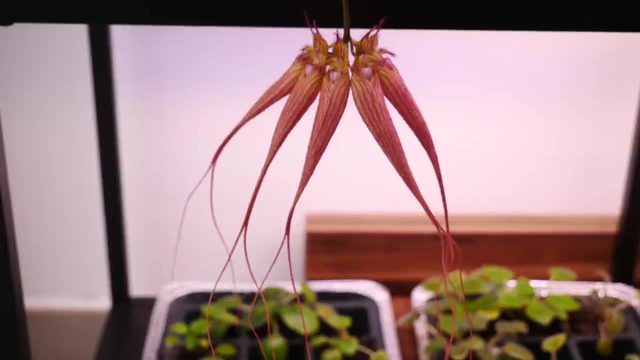 need a lot of humidity and all sorts of special things that you cannot implement in a home you will not find in this video. To me, Bulbophyllums are the thirstier version of the Phalaenopsis, if you will, At the 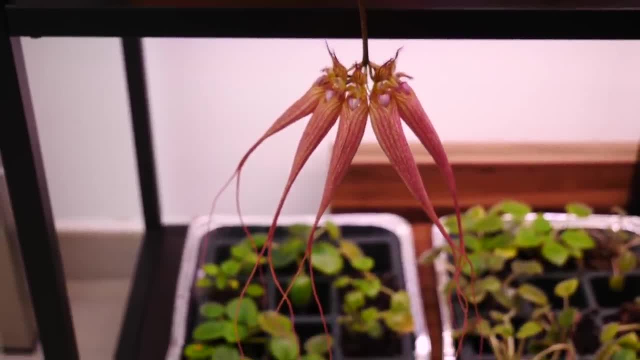 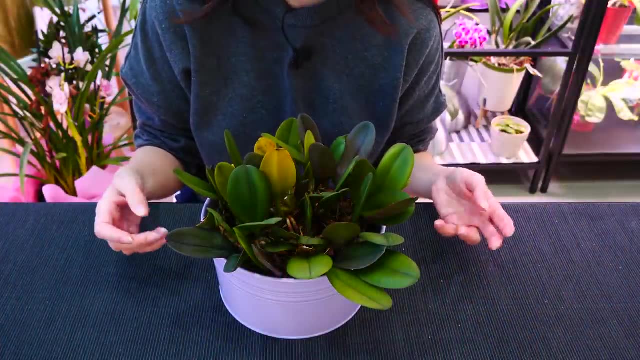 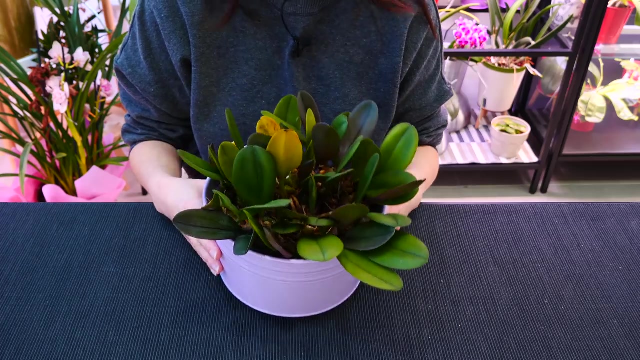 same time, though, they don't tend to bloom as often and as long lasting as Phalaenopsis. They don't necessarily have the most interesting leaves either, and certainly they can grow out of hand because they are a crawling type of an orchid, It is a sympodial and it has quite a long rhizome. 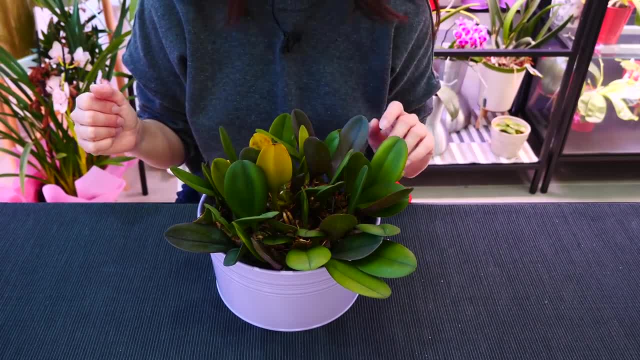 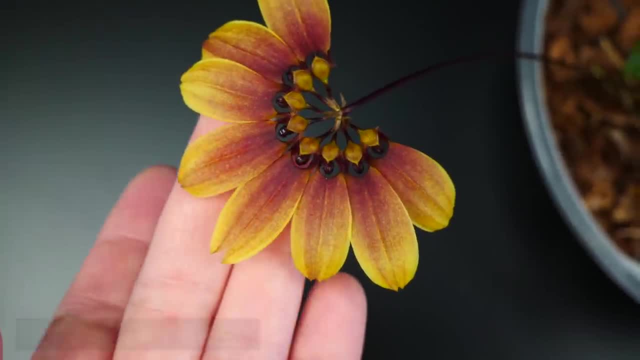 There are exceptions, obviously, but the one that I'm going to talk about today is the Phalaenopsis, The ones that I have. they are naughty. They tend to spread really fast, So that is a drawback Plus. the fact that you don't see it in bloom all that often again is a drawback Plus. some of 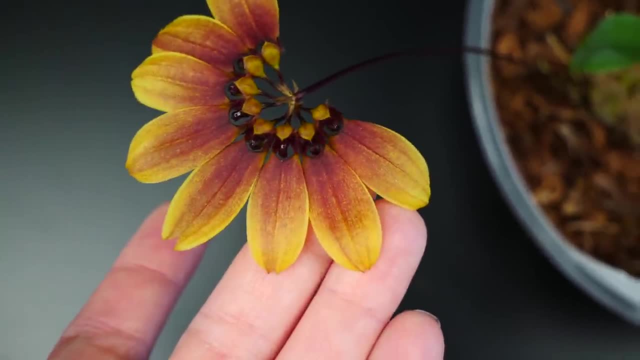 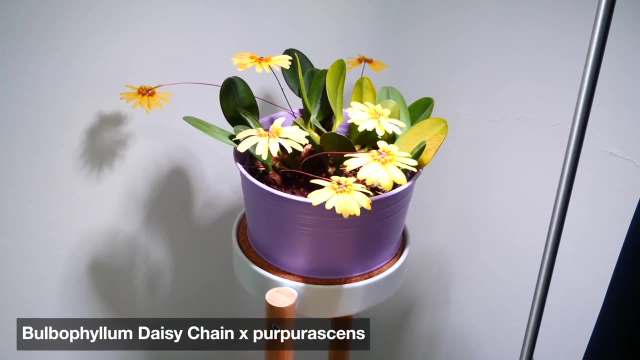 them smell really bad, Like really bad. Their pollinators are flies You can't imagine, But they're just so beautiful and so easy to take care of once you get the hang of things. They're just not as easy to bounce back. In my experience, all of the Bulbophyllums that I ever lost except one. 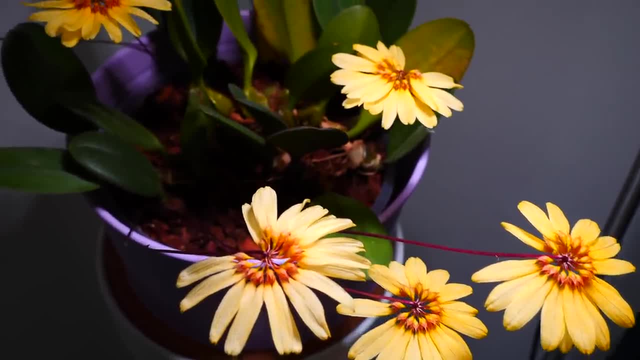 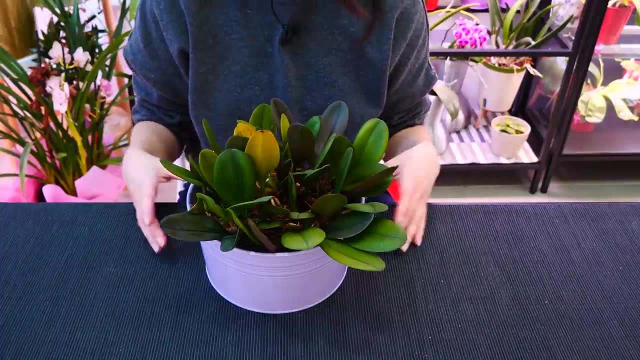 which I think had a virus, but all the others I think they are the most beautiful and the most. I lost them because they had a rough transport or they weren't very healthy to begin with, And rehabilitating them it was not easy, So that's the only drawback that I see with Bulbos. 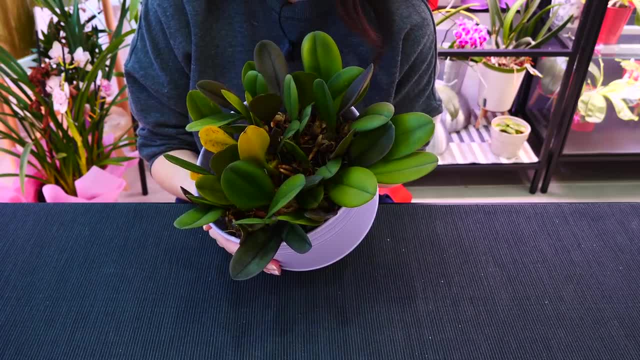 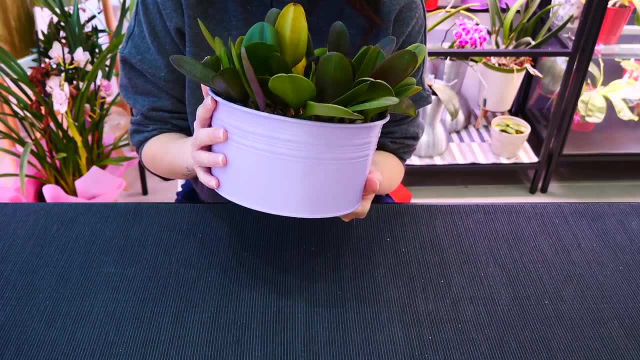 They're quite sensitive when it comes to almost losing them, But other than that, once they get going- look at this guy- They're really easy to grow. They don't require a lot of light, but they don't bloom as often either. However, I just find them a joy to grow in a home. 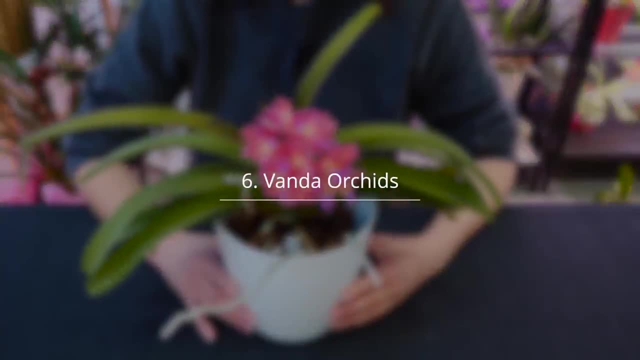 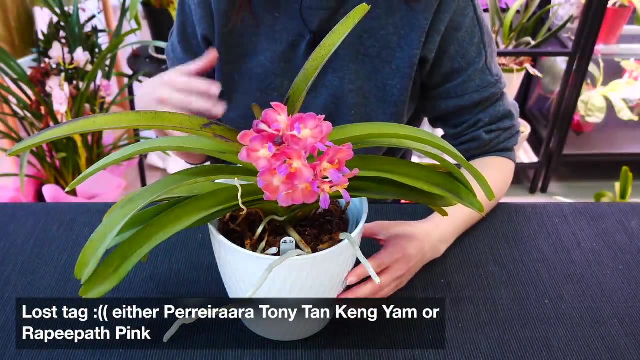 Next up it's got to be Vandas. for me, Oh man, Vandas. I think I'm on a mission to popularize Vandas together with the Bulbophyllums I don't under. I mean, I understand why they're not as popular as Phals, But don't they look like? 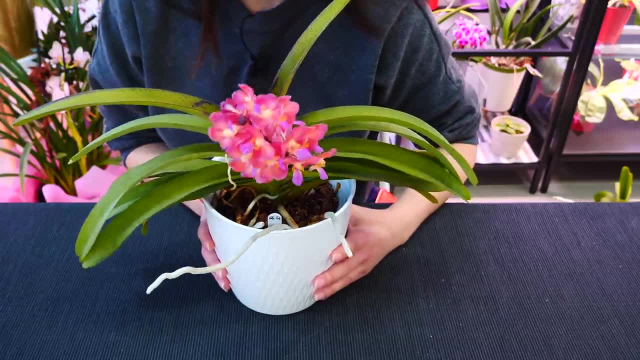 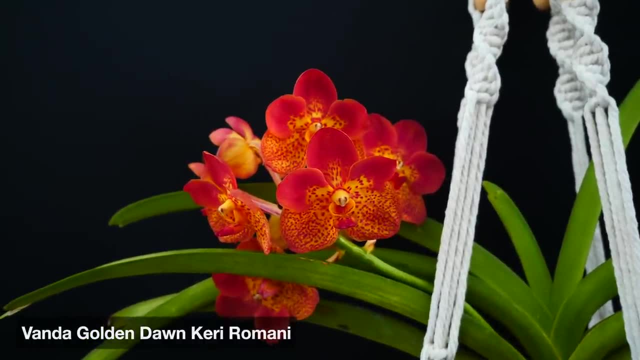 another type of Phalaenopsis, Kind of right. Well, Vandas, I believe, are not as popular because they are sold bare-rooted And it's a little bit intimidating If you think Phalaenopsis are intimidating because they're potted in transparent pots and they have roots everywhere. 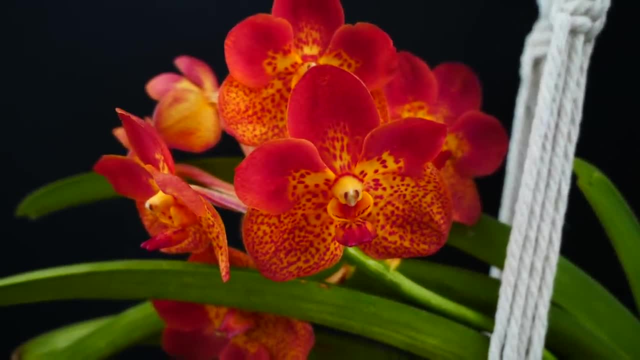 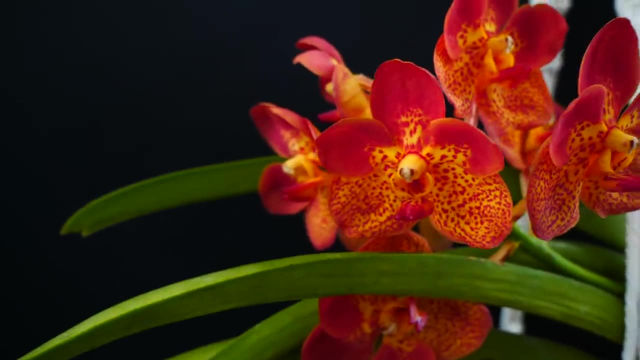 imagine a bare-rooted Vanda. Yeah, it is intimidating And it is quite the large. But on the market, in nurseries, there are tiny Vandas available as well, And if you manage to acclimate them to pot culture, it's going to be much. 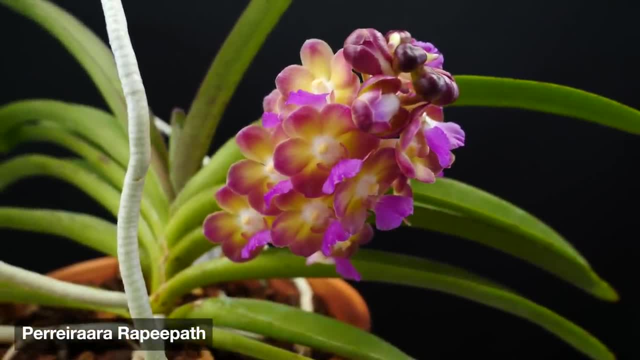 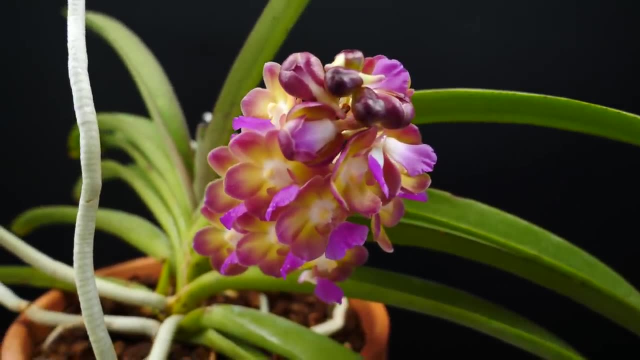 much easier to take care of something like this in a home. I do have a video on VandaCare, just like any other orchid down below, But I also have a video on how I like to switch them to pots. It's not an easy process, depending where you purchase your orchid- Sometimes from some 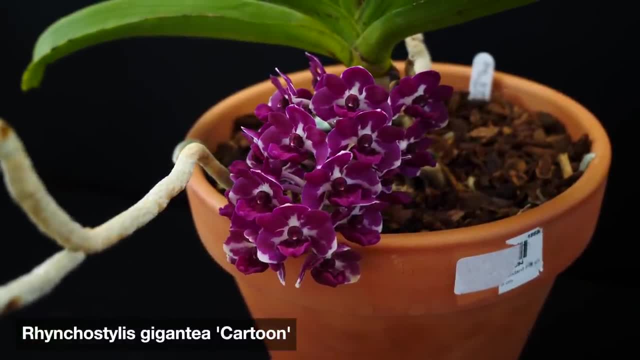 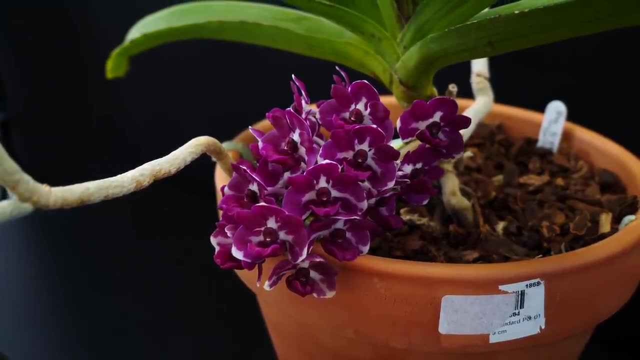 potting Vandas, But it was kind of rare. But the market is changing. If you get a Vanda acclimated to a pot, great, I don't think it's way different than a Phalaenopsis. Yes, it does require much. 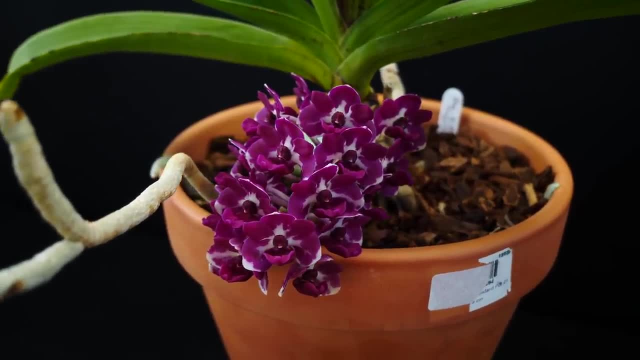 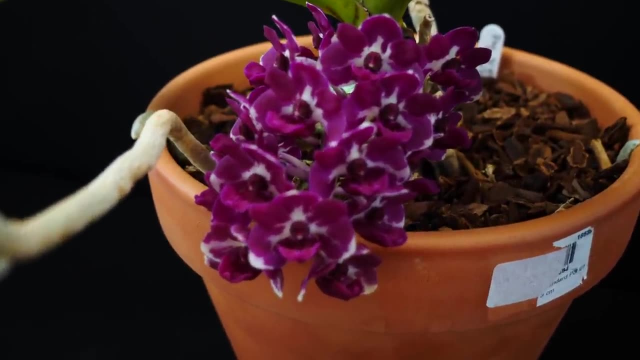 more light And yes, it is a hot grower But it doesn't need that cool down to bloom And it can also stay pretty small if you choose a variety that stays small. But for me Vandas are high up because I did manage to adjust all of my Vandas to pot culture And 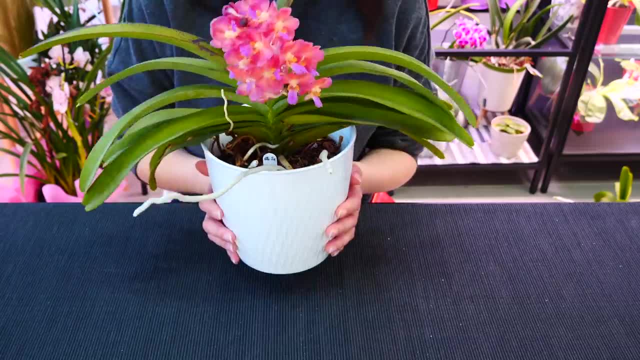 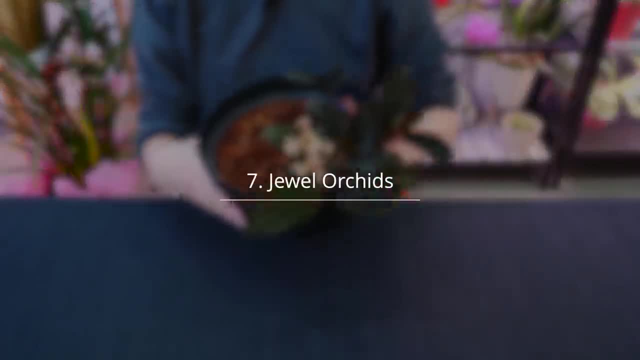 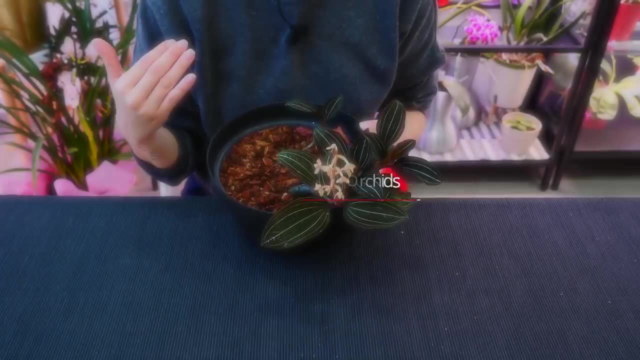 I have a great time with keeping them like that in my home, So definitely give Vandas a chance, because I think they are beautiful. Next up on the list is jewel orchids. Now I would put the Laodicea discolor further up in my list, maybe as close as Phalaenopsis. 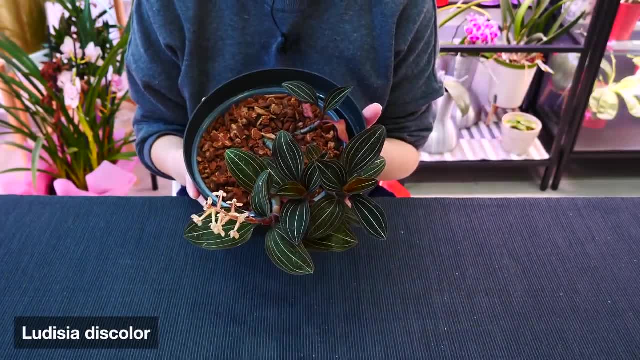 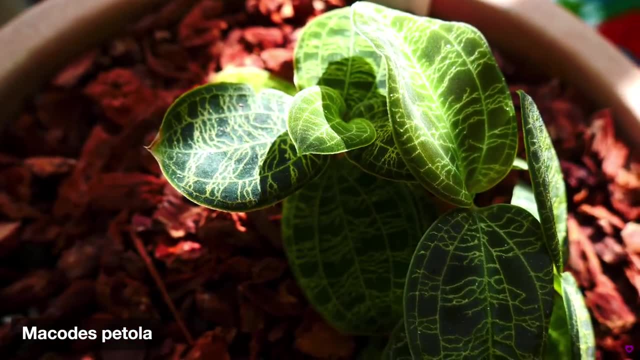 But I will keep it here because Laodicea is not the only jewel orchid we can grow And other jewel orchids are just a little bit more finicky, slower growing, not as friendly, Quite intimidating. So because Laodicea and its hybrids are so easy to grow, they don't demand. 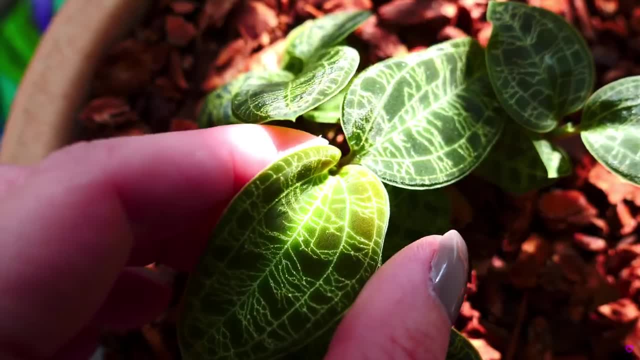 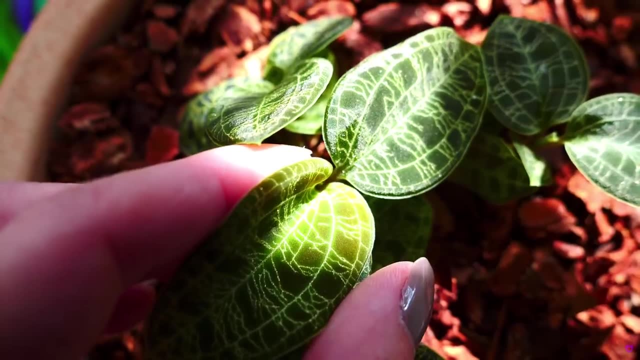 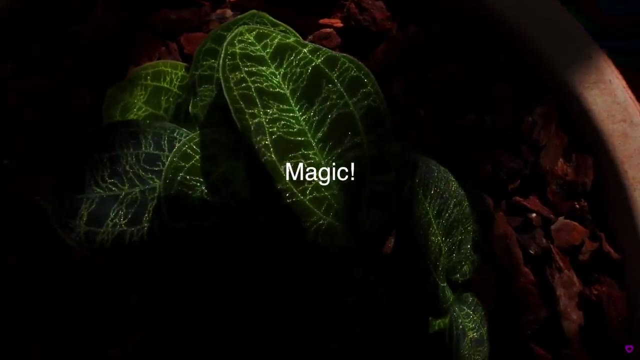 a lot of light. They just grow in whatever type of soil you have. For that reason they are here. But other orchids might demand a little bit of a higher humidity to grow well, although they can grow well in a home as well. But I don't know if you have a very dry home. If you do, if you. 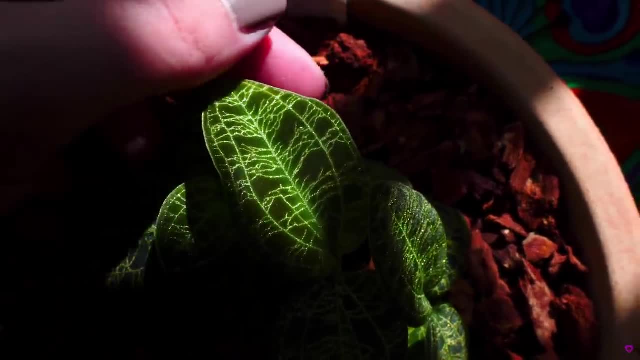 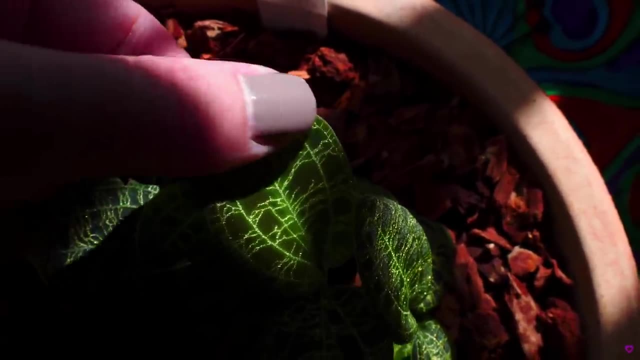 struggle with humidity. you might struggle with some of these guys, So it's hard to generalize. Laodicea discolor is easy and I do believe it will do pretty good in almost any type of home, But because there are some individuals that really don't like certain environments, I'm just going 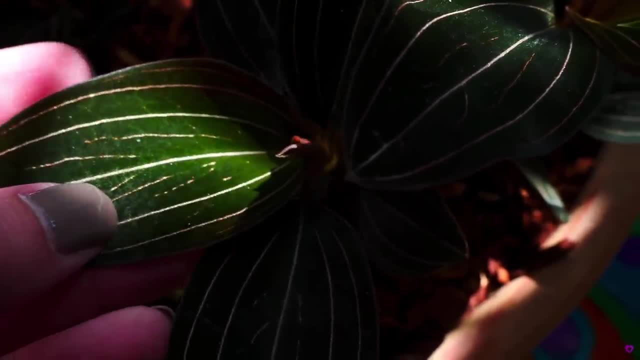 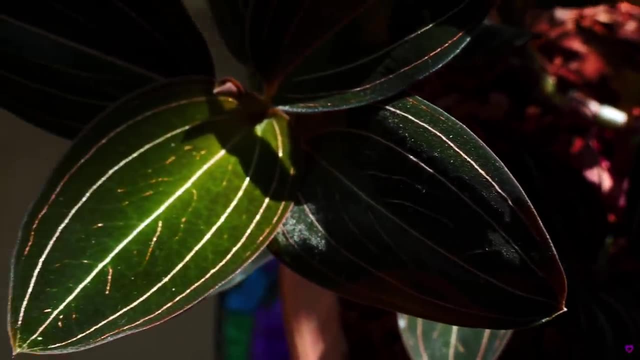 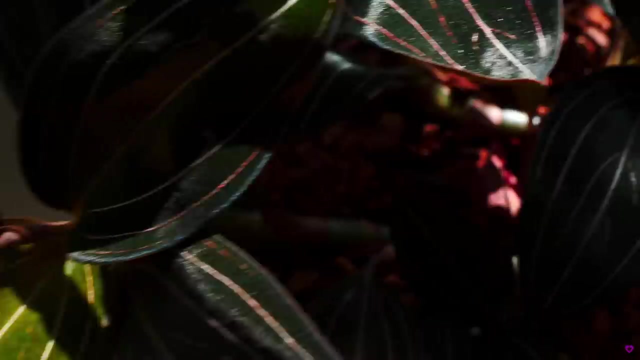 to keep it here, I have a tutorial that I recently made on jewel orchids and Laodiceas. It's hard to generalize. I might think that maybe the Makotas will be difficult for some of you, but turns out it's not. I might say, oh, this is super easy to grow, but you might not have. 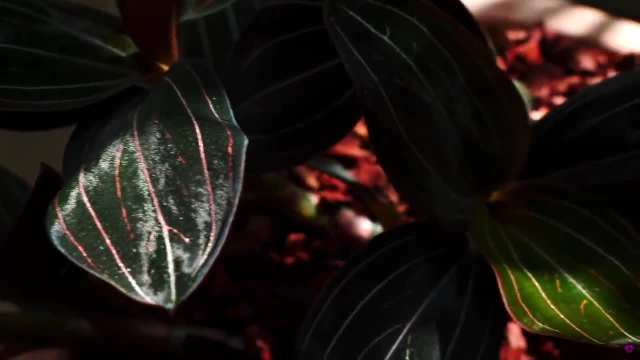 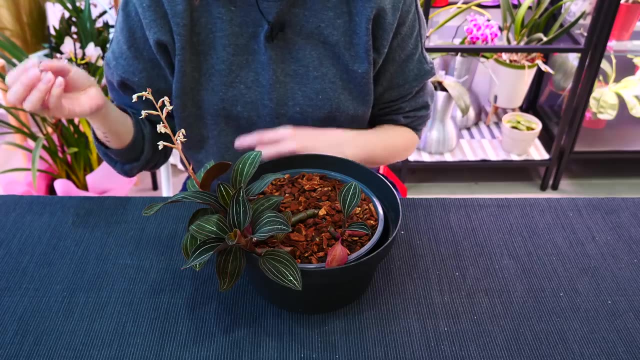 good success with it. It really depends on environment, So I'm not going to put it high on the list. I'm going to put it in the middle. I consider it to be easy, but I can see how some people can struggle with some individuals of this particular family. Next up: telumnia orchids. 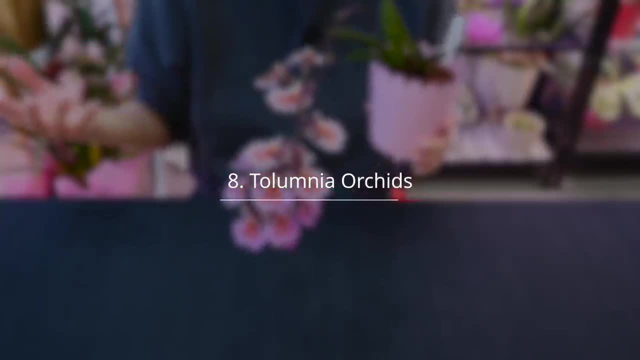 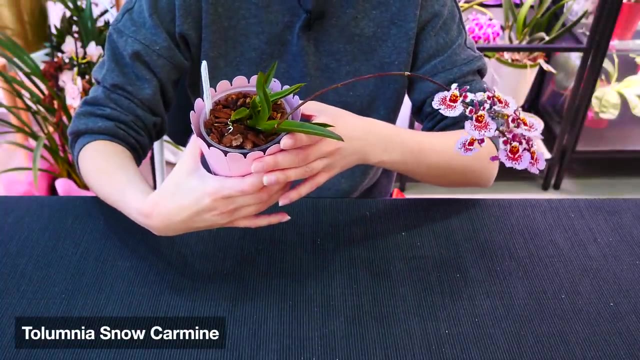 Again, I feel they're not as popular as they should be because they're not all that available in flower shops across the world. But telumnias, I believe they're great for home growing because they're rather tiny And look at this flower display. Typically on telumnias you'll have 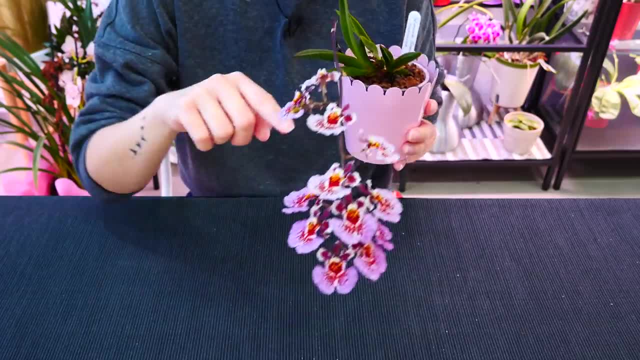 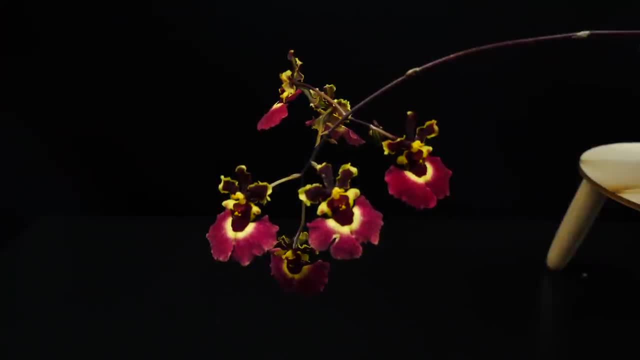 bigger flower displays than the orchids themselves. The flowers look like oncidium flowers. They're not fragrant, typically, but they are just so charming, And a telumnia can bloom multiple times a year. You don't need to drop the temperature or anything. You don't need high. 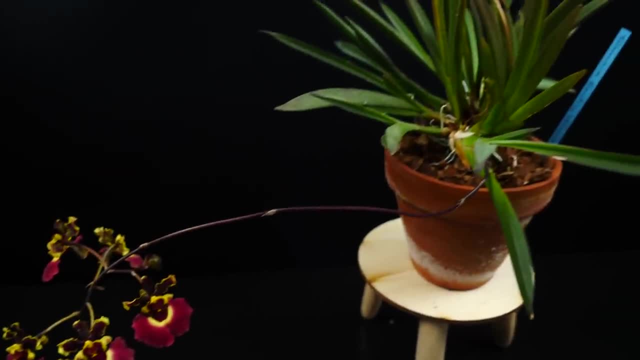 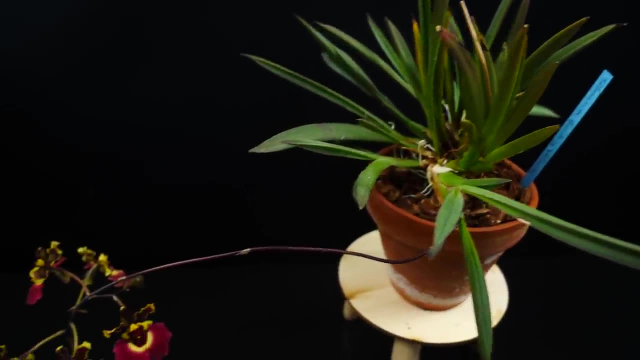 humidity. Again, you don't need greenhouse conditions to grow these guys. Where I think the downfall is with telumnias, is getting the mixture right. These like moisture, but they like air just as much. So with your mixture you need to strike a balance. 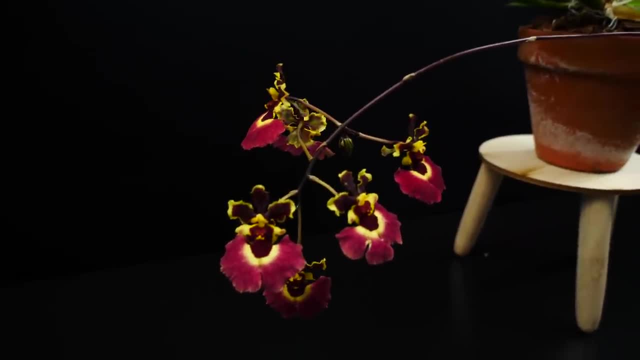 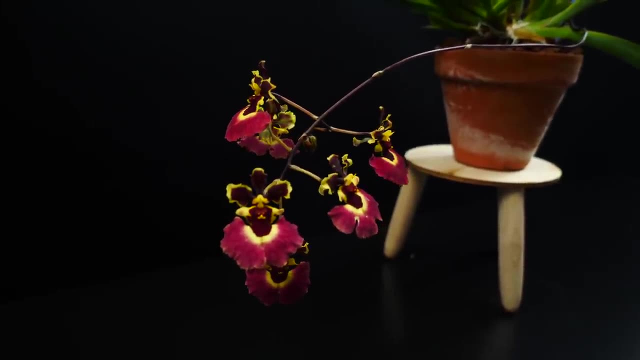 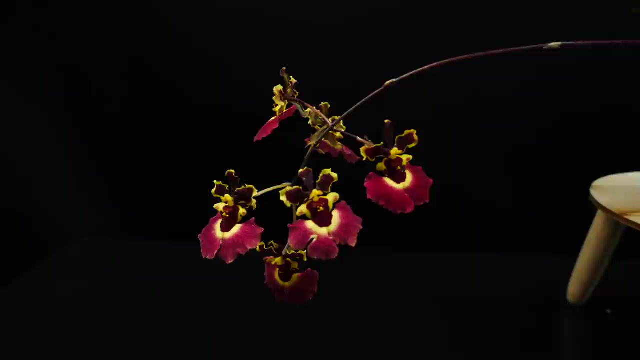 between having a lot of aeration and keeping them hydrated. I don't feel like telumnias are drought tolerant. Whenever I skip watering day I start to see little wrinkles. So I need to water. But if I make too much of a wet- let's say mixture, too much sphagnum moss, that's not really. to their liking. They grow much better when I offer a lot of ventilation and a lot of moisture at the same time. So it can be a little tricky to find the proper mix, But once you do, I don't think you're going to have a lot of issues. Another thing that they're not great at: 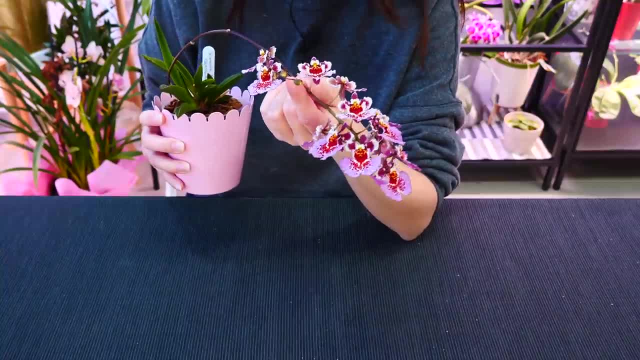 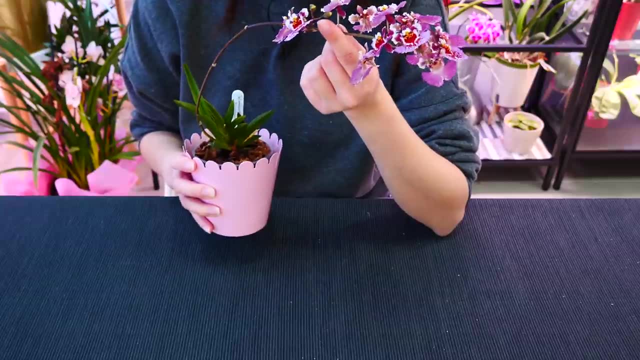 is bouncing back fast. A setback. telumnia can definitely bounce back, but it's going to take a while. All of mine that were in bad shape due to I don't know, transport, wood loss, battery potting and things of the sorts. They took a while to bounce back. A while For a tiny. 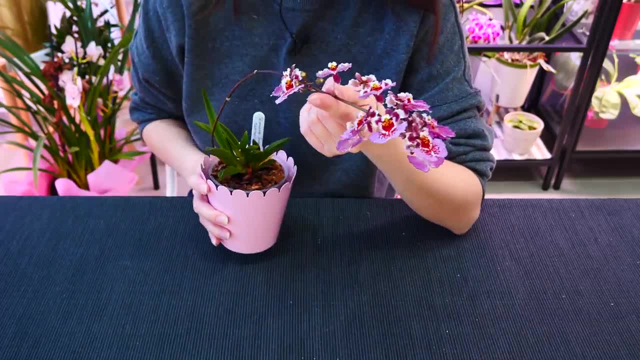 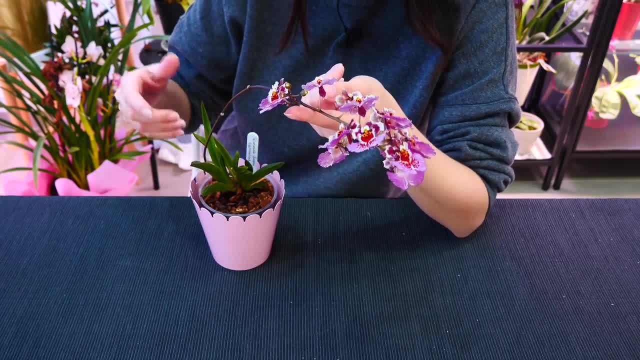 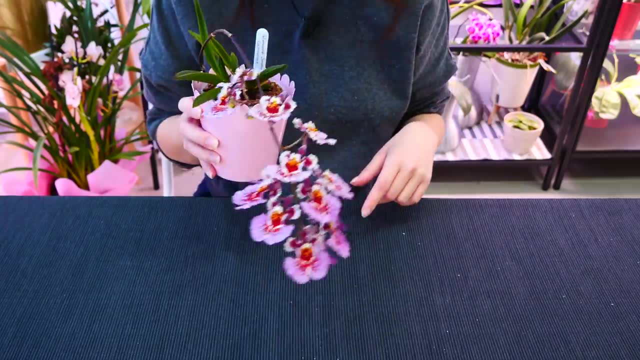 No, It takes a while. You'd think you know that it will bounce back fast because it has fleshy leaves, It has reserves. No, It takes a long time, I don't know why, But once it gets going it's great. So, because of the reward and the very little space they take, I will put telumnia. 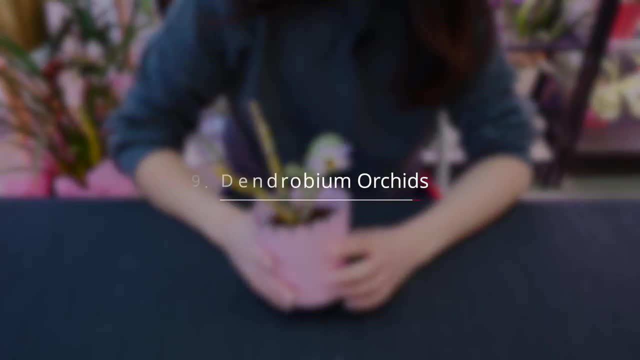 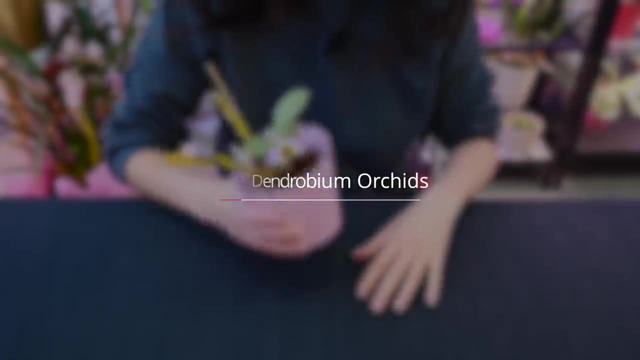 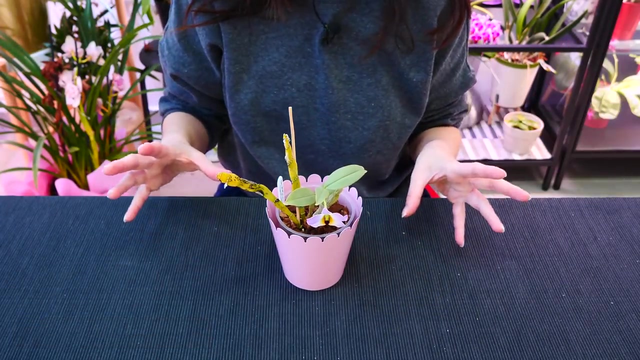 somewhere in the middle of my chart Next up, I'm going to place on the list dendrobiums, generally speaking, except the noblies. Noblies are further down, But dendrobiums are just such a varied group of orchids it's just hard to split them in all sorts of sections. 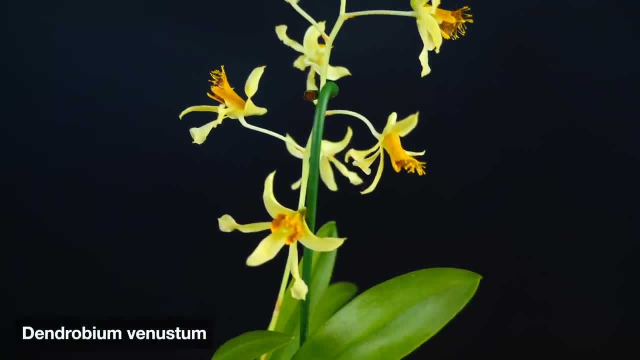 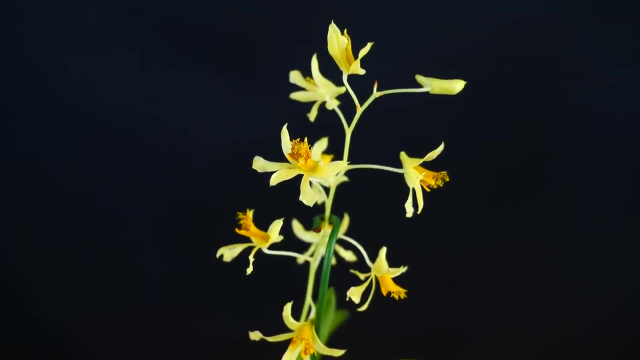 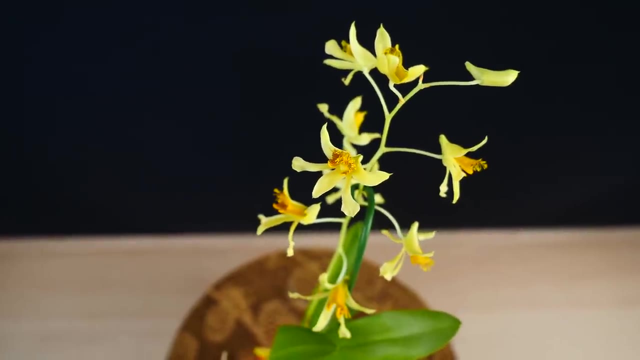 So I'm just going to bunch all of the dendrobiums together at this stage of my list, because there are some which are more finicky than others, some that are not really finicky at all, easy to grow in a home, but they're pest collectors. Generally, dendrobiums are known for really attracting pests. 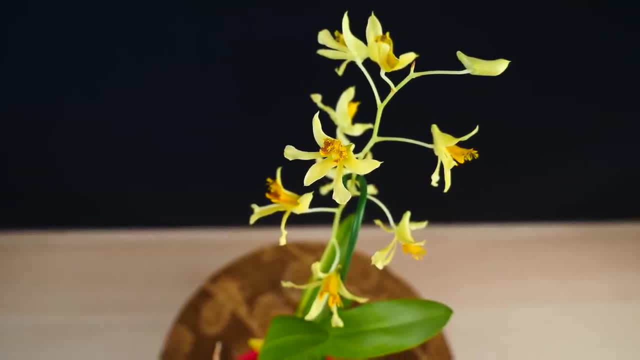 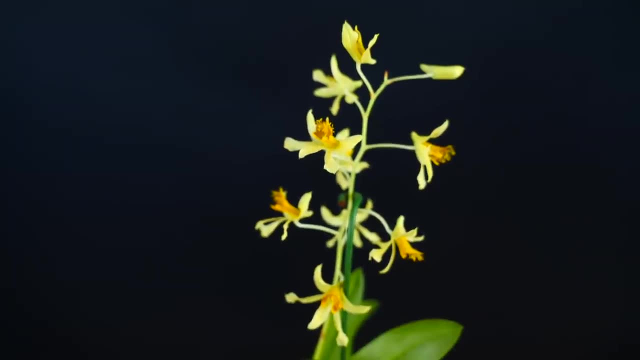 which is not a good sign. Some dendrobiums do take a little bit of a winter rest, but it's not like the Phalaenopsis. You don't necessarily need to drop temperatures, in my opinion. again, except the noblies, Some are deciduous. I'm not sure how many people like to have bear canes in. 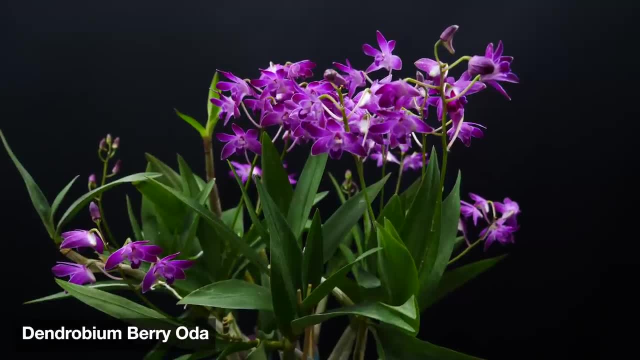 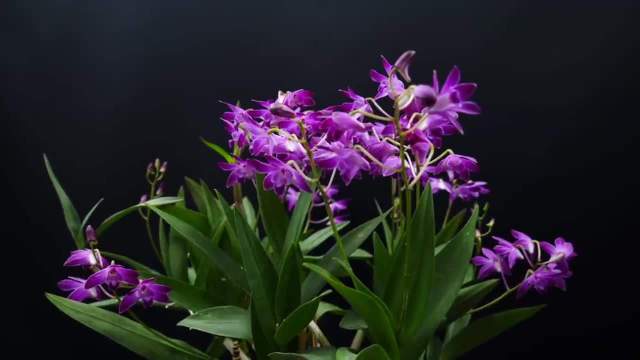 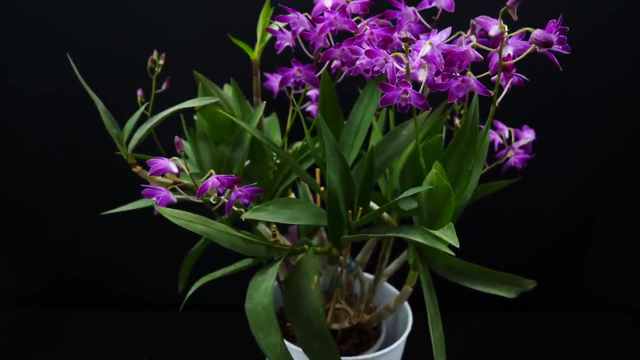 the middle of winter, with nothing on them And just to wait for a once-a-year show? you know maybe not what you would want. Some dendrobiums are big. some are absolutely worth it and easy to grow, like the Baryoda, I think it's very easy to grow. Some are just not very easy to grow. So because 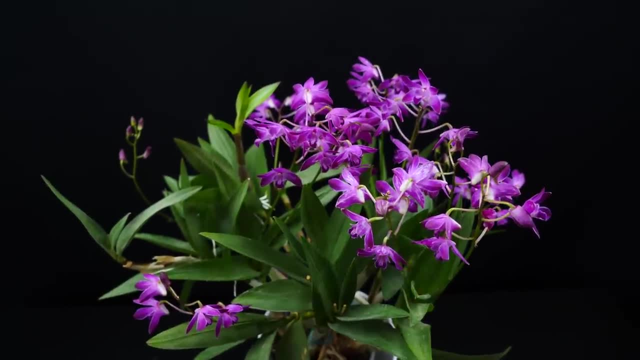 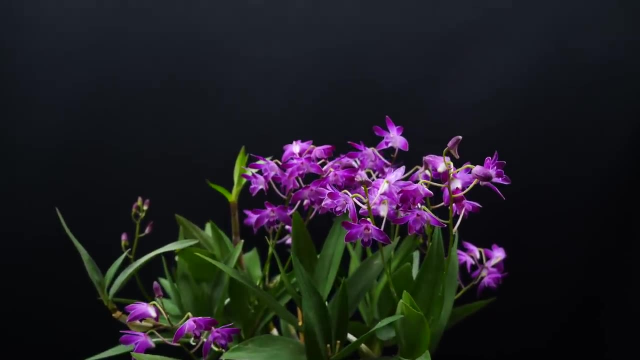 of that. you kind of need to pick which one you think will do okay for you, which one you have more available in your area. But generally speaking I find dendrobiums to be somewhat on the lower side. They're not the most finicky orchids for me generally, but they're not the 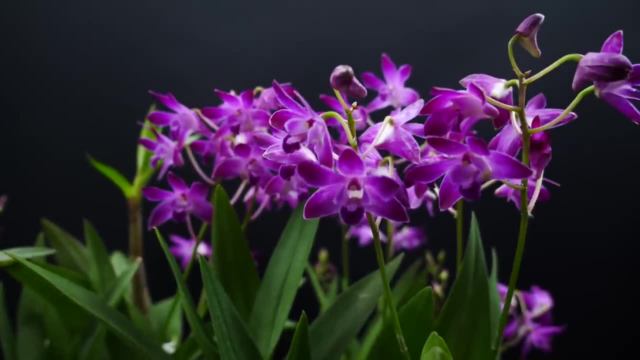 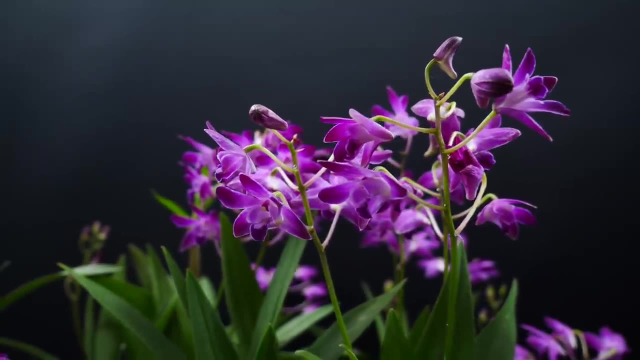 most glorious either. I mean my fowls and my cats are glorious, not these guys, but I do okay with some of them, So that's why you don't see a lot of dendrobiums on my channel. I'm not a fan of stuff. 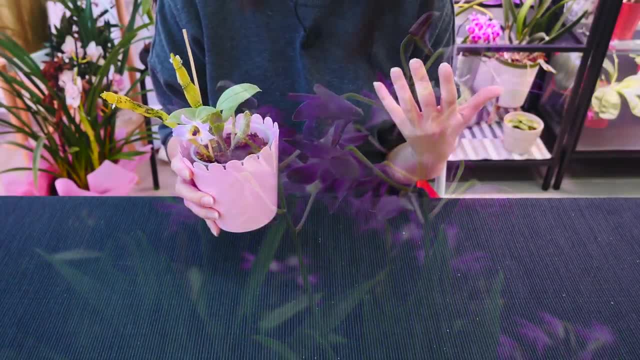 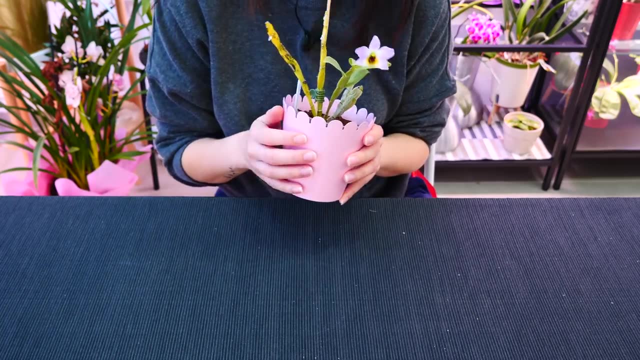 that are just not happy with my fowl. You know, if they don't like me, you know I don't want to keep them here by force. So I don't have a lot of them and the ones that I do I really like or I think they will do okay. 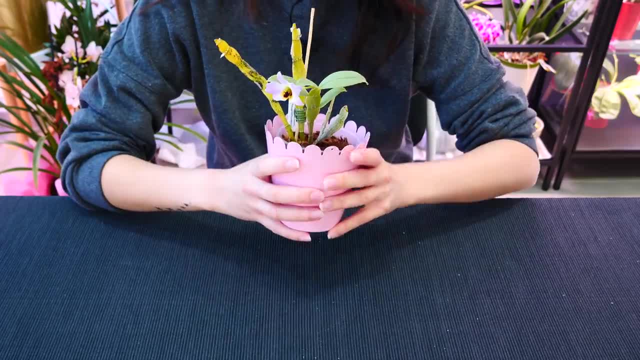 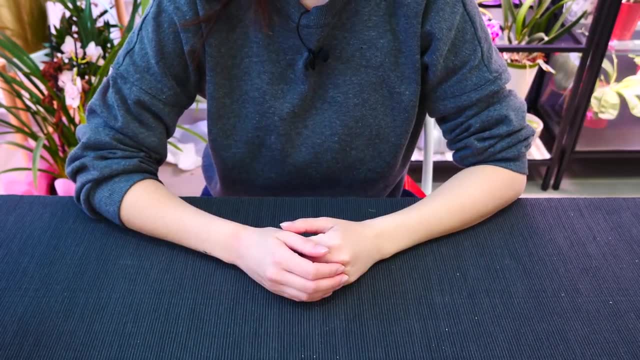 in my environment. So for me, dendrobiums are here on the list, bottom of the list, but not the most bottom position, Dendrobium nobilis. on the other hand, oh boy, where do I start If I? 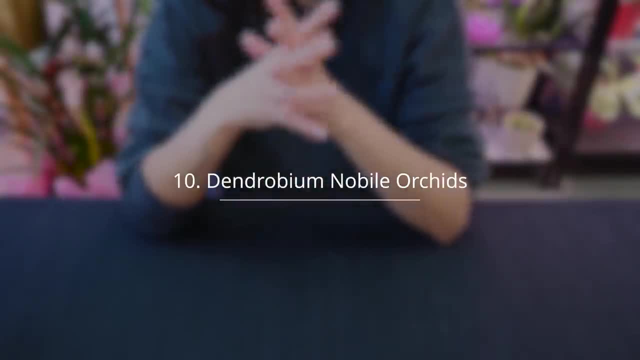 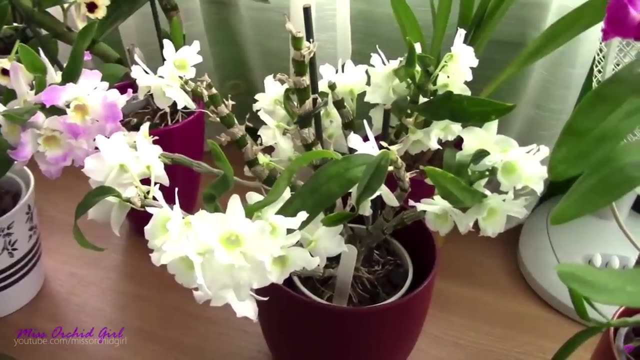 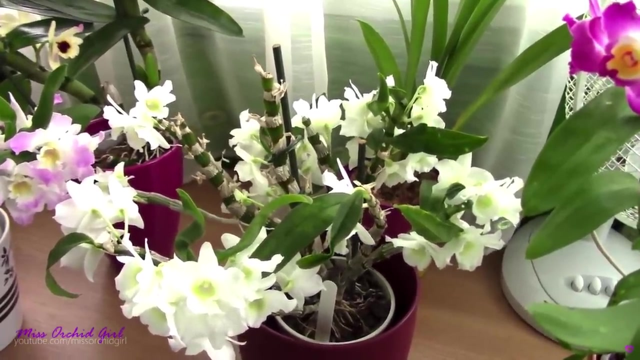 would be living back in Romania in a temperate climate. I would say. dendrobium nobilis are easy. they have beautiful plants, but now that I live in this subtropical climate I cannot Like. they have such a specific pattern of growth that I don't get it right Mid-season winter. 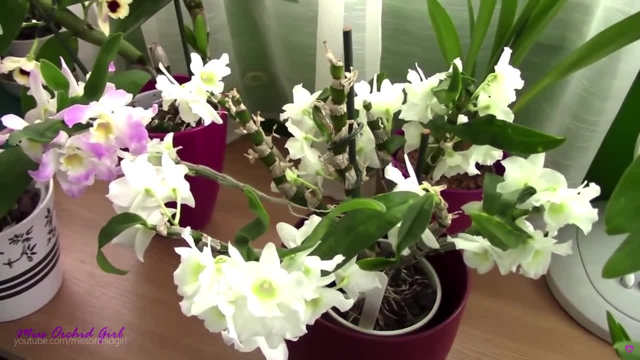 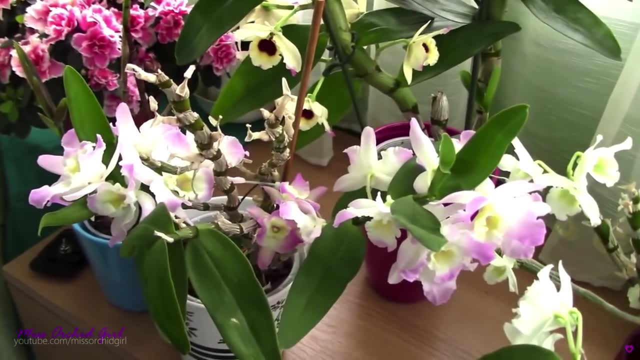 comes. they're midway through their growth, the second growth because, yes, they grow two growths in my environment, because I have long summers, And then they just end up depleting themselves, trying to figure out what type of season it is. what they should do, should they bloom? 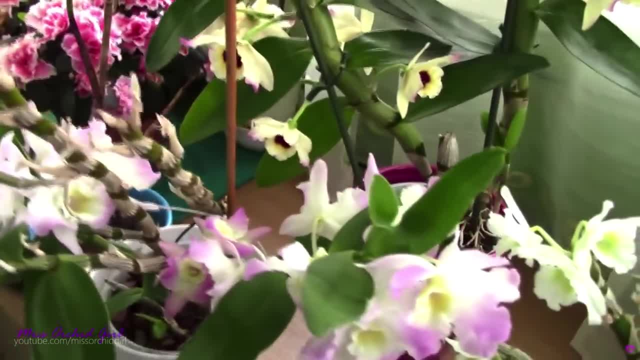 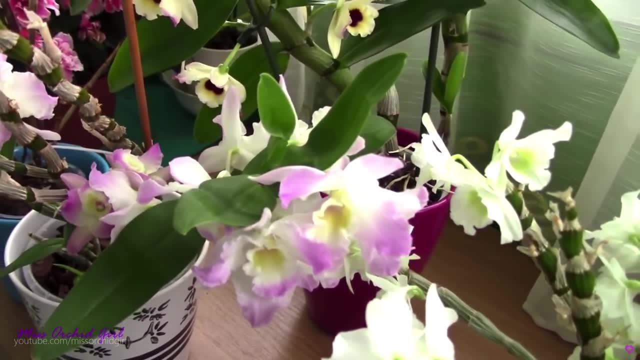 should they not All of that drama? I talked about it. It's not worth it. So, with dendrobium nobilis, on my personal list they're low, but on other people's lists they might be higher up, because if you have that particular climate, 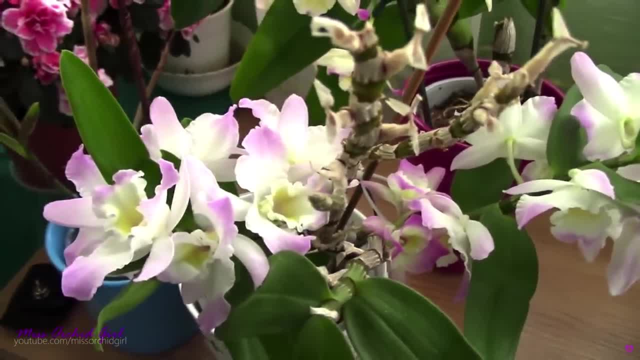 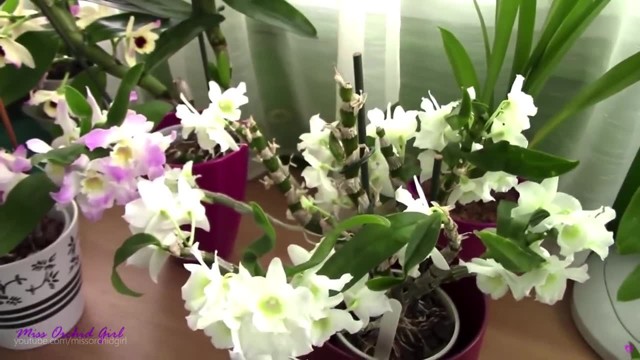 that helps them out. it's great, It's fantastic. They're beautiful. They smell nice. You should definitely own them. They're not finicky at all. They can grow in a home. You just need to pay attention to the winter rest And other than that, they should be absolutely fine And for the time, 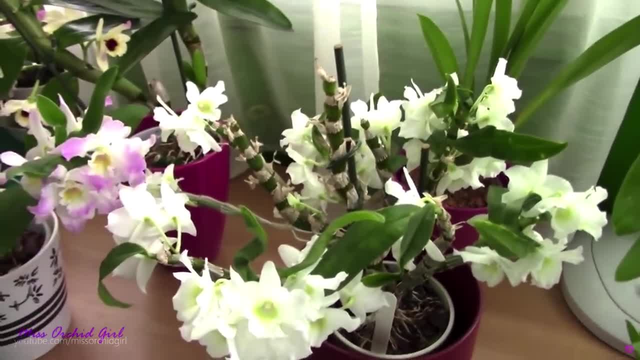 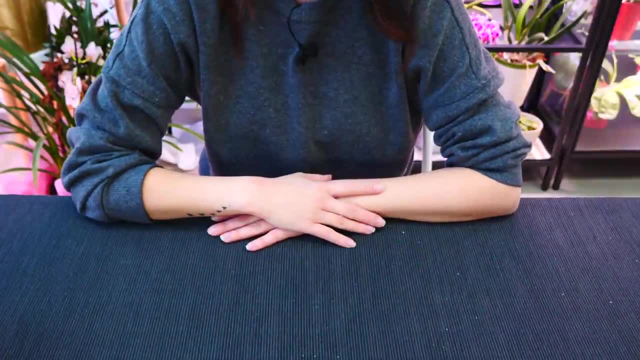 that I grew them in Romania. I had no issues, no issues. They were the easiest. Well, things don't sit the same way here. So for me personally, they're low on my list. I don't even bother purchasing them anymore. I don't know if I will ever purchase them, If I have one. 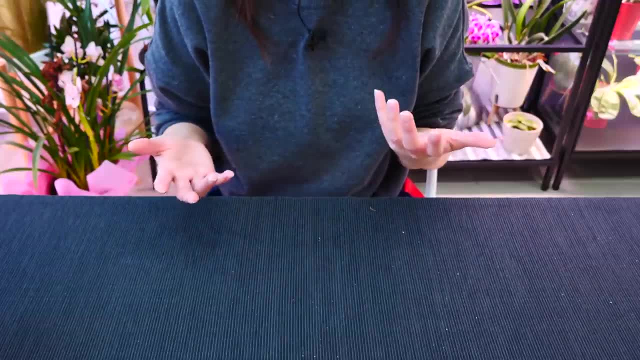 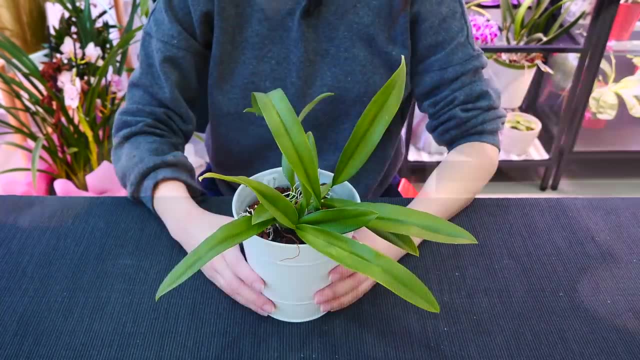 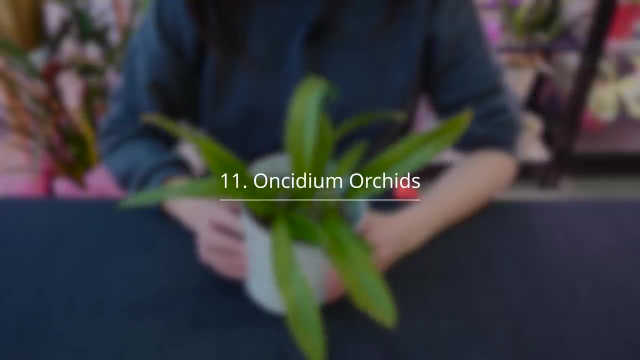 maybe I'm going to get it for a video or for an experiment, but I don't want to lie to myself. I can't grow these guys anymore And that is that All right. Are we ready for the bottom of the chart? Yes, Oncidiums. I can't believe I'm putting them on the bottom because I love them, but oh man. 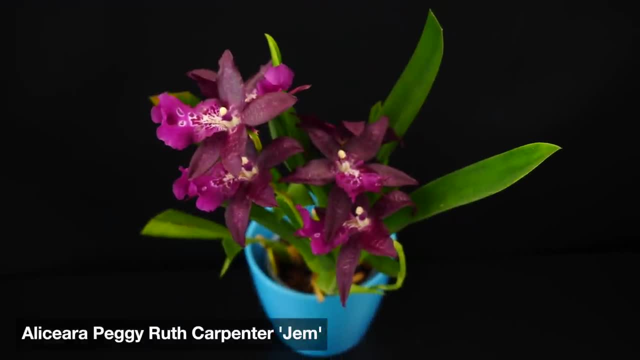 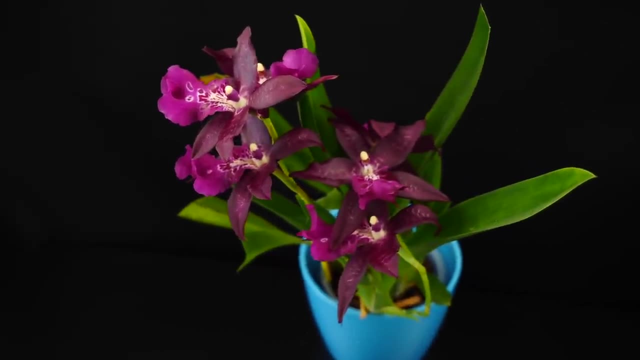 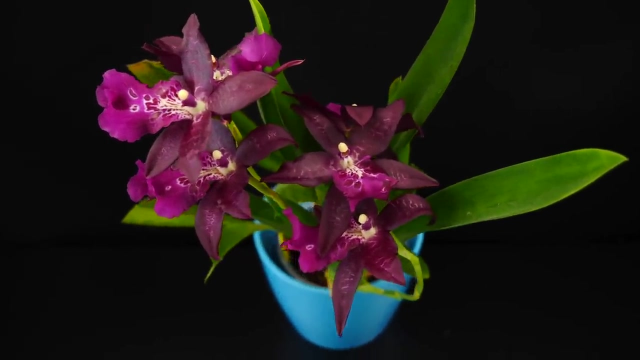 considering the last year that I had with them and how many I lost due to the pest infestation, I can't, I can't. So oncidiums generally are easy to keep. They are not very demanding. You can grow them in a home. They have been the first serious, let's say orchids that I managed to save. I kind. 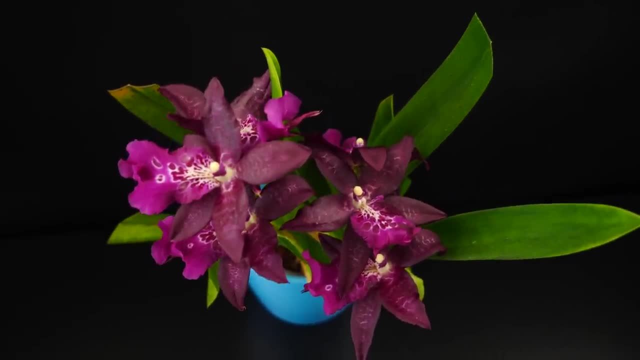 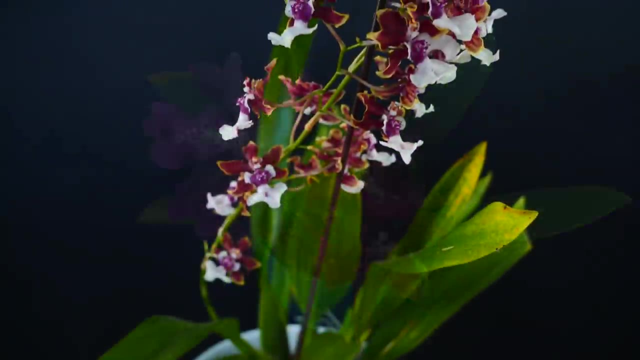 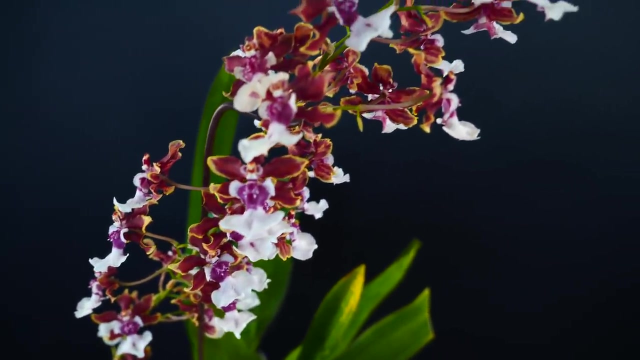 of built my foundation knowledge of orchids on oncidiums, because I purchased a lot of them discounted dirt cheap, like nine years ago or 10 years ago. So I built my channel and I built my knowledge on oncidiums. I know a lot about them. This being said, when it rains, it pours. 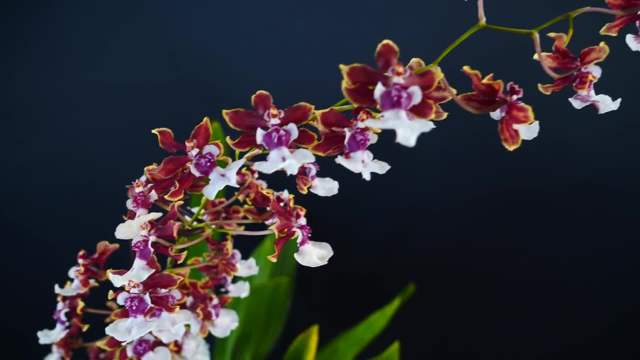 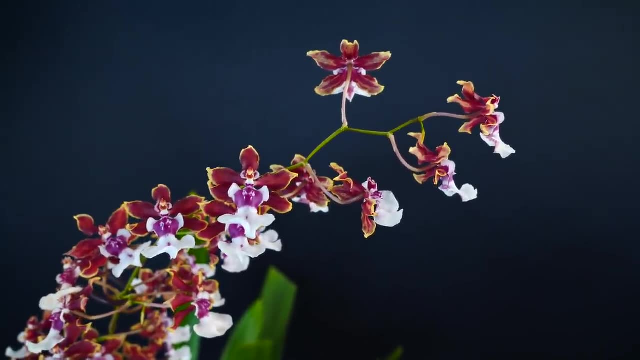 with them when things go bad. oh man, they roll so fast if you don't have time for them. So these guys should be really easy for a home grower. If you don't have a lot of orchids, they will be very. 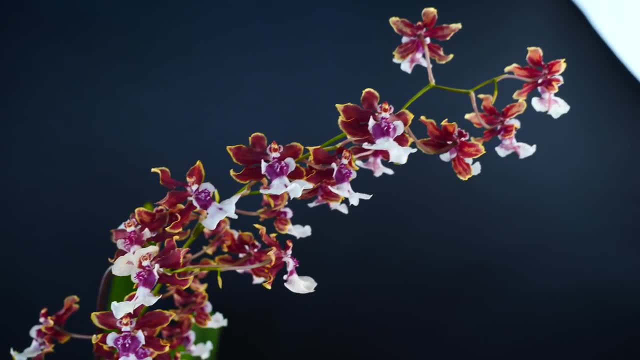 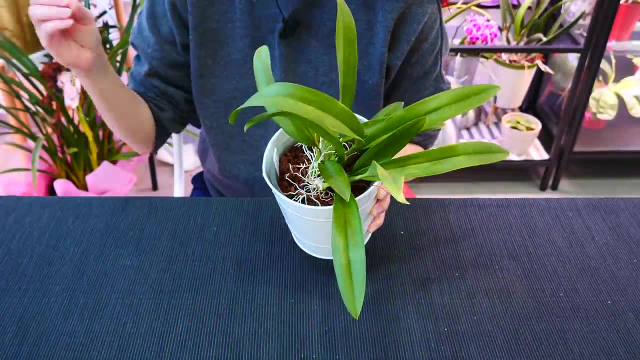 easy, But if you have a lot of orchids, maintaining these guys will be a nightmare. It has been for me. I am definitely never going to purchase as many on the stadiums unless I have a contingency plan, but I have a lot of work to do. 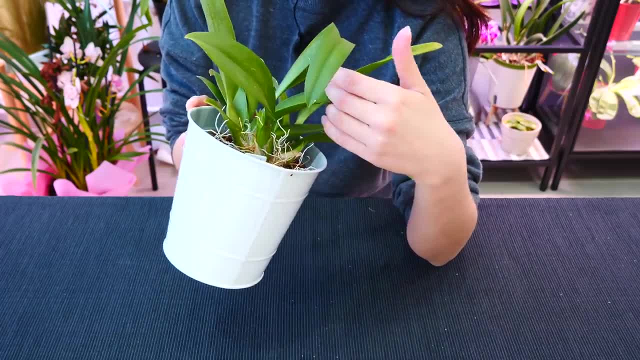 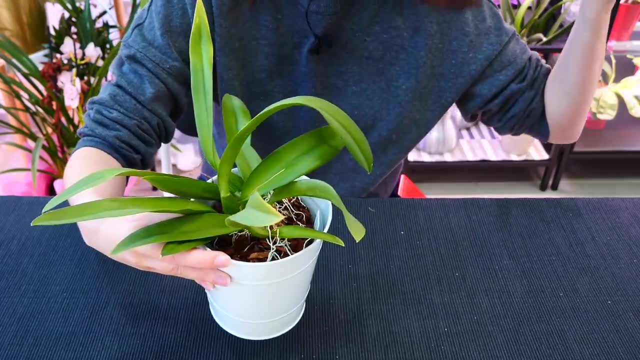 happens is because they have these growths which are kind of like an onion, they have a lot of layers, and because they have big leaves. i'm showing you a tiny one, by the way. there are others that are big. they have a lot of leaves. they're very foliage oriented plants. they have leaves, they have. 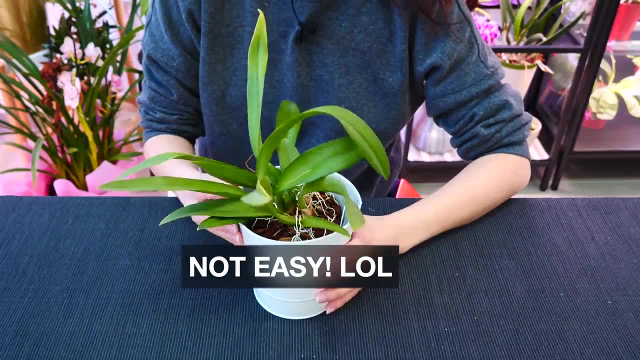 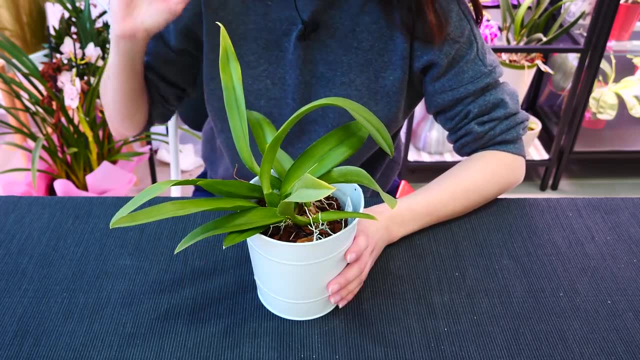 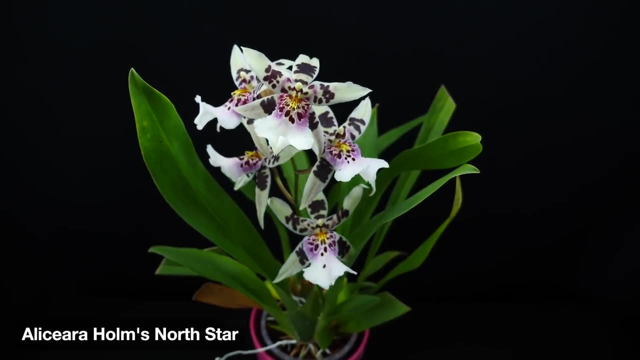 pseudobulbs. they have large structures. it's easy to contain a pest outbreak. you might contain it on the surface. you're gonna break your bag. it's gonna take a while. if you're not using, let's say, toxic systemic means. if you're using spot treatment, let's say, oil-based solutions, it's 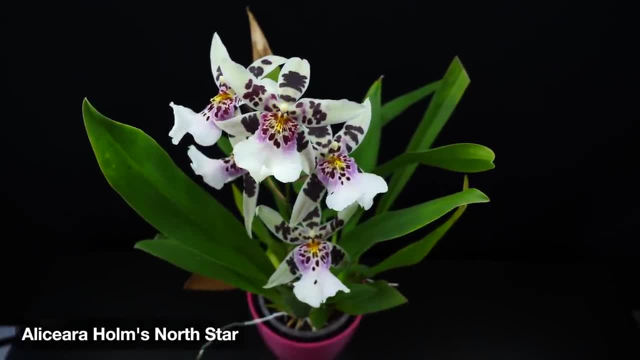 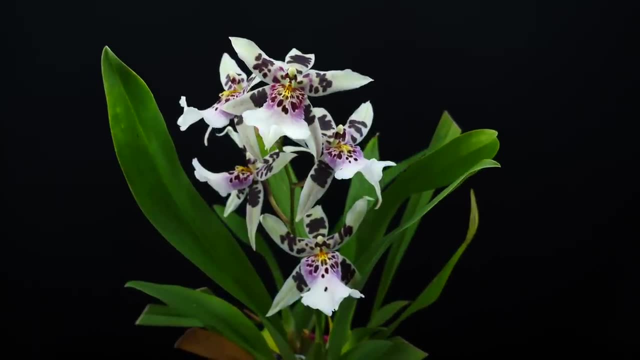 gonna take an eternity, it's gonna break your back and you're not gonna achieve success. necessarily because- oh, look at that- the pest might hide themselves in the new growth. can you do anything about it? no, because if you put water in the new growth it's probably going to rot. can you oil it? 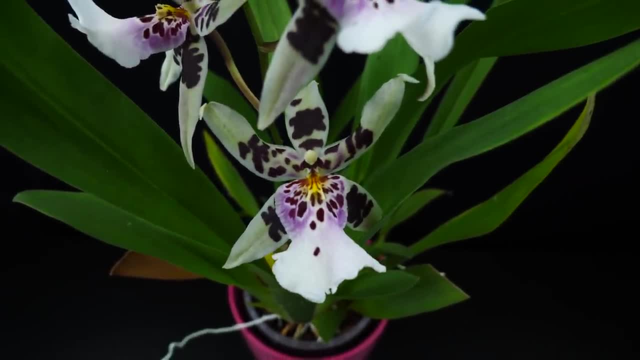 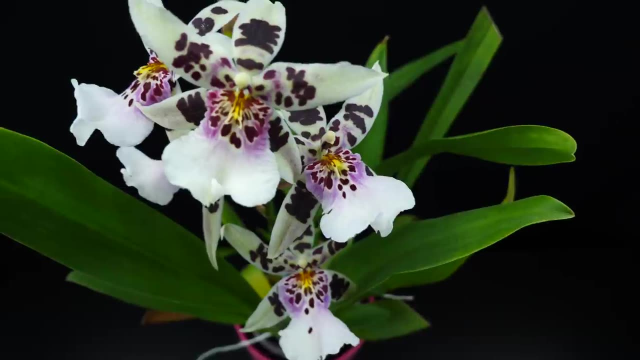 really bad? no, because the new growth is pretty tender and you're gonna rot it again. it's not a pretty situation if you let a pest outbreak get out of hand, and with onsytiums it's really easy to do so. whenever we grow our kids, we need to be a little. 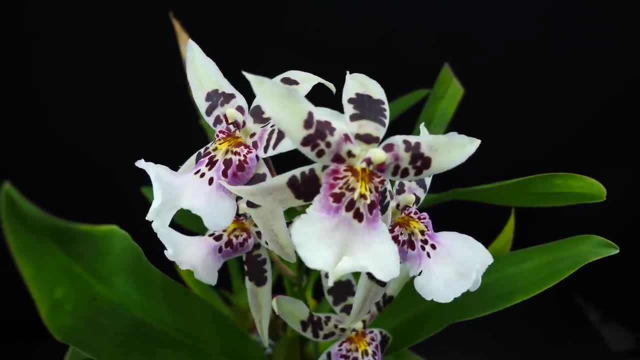 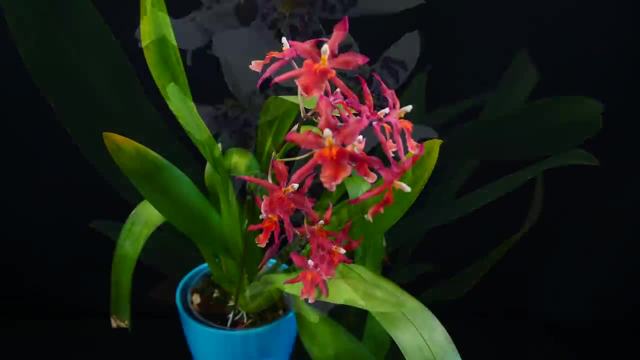 realistic. yes, we have time for everything now, but there might be a time in our life when we need to focus on very important stuff and neglect some parts of our lives which are not all that important. it's not because we want to, it's because we are forced to right. so this is the reality of things. 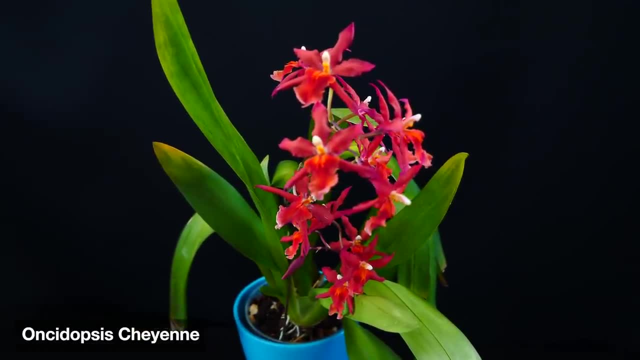 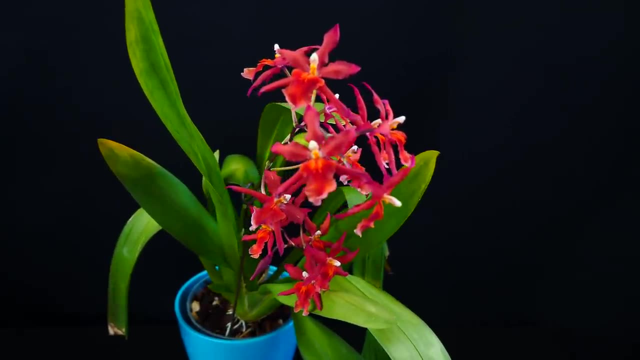 the first ones to be affected by neglect, i think, will be onsytiums or onsytium types. i'm going to include here the meltoniopsis as well: meltonias, brassias, even zygoteas, and then the other ones. 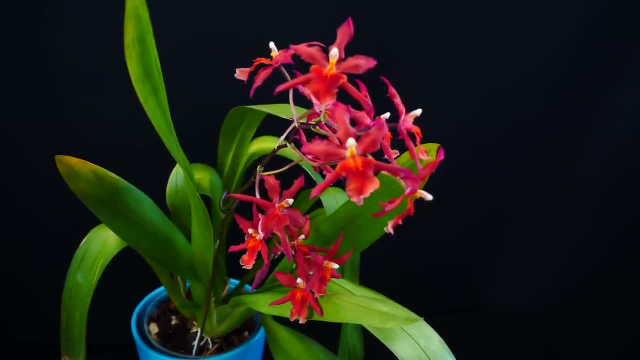 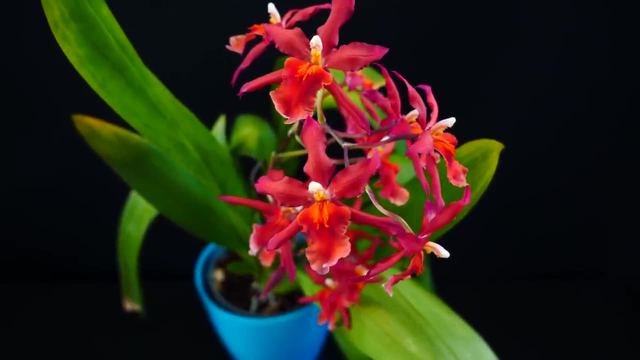 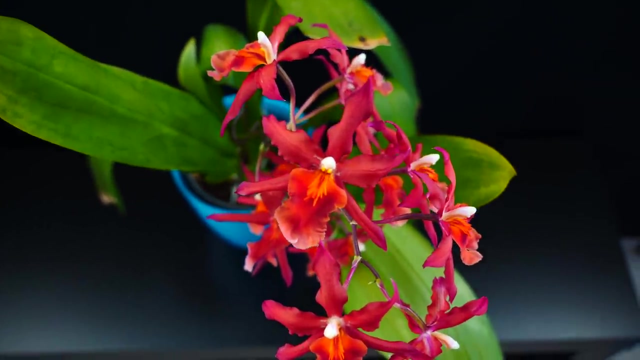 i'm going to include them as well. all of these guys. i think they will take the hits in your collection and when it comes to rehabilitating them from a pest infestation, it's gonna be a long, long hard process. that has been my experience with them- and sad because i love.